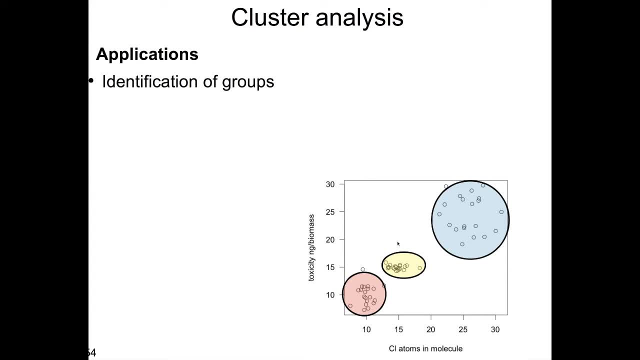 So what are the applications of cluster analysis? First of all, just the identification, The identification of groups, as already mentioned. The second objective is then to aggregate data. You have a dimension reduction, like for ordination methods, because you could replace the membership, the individual observation, by the membership to a group and use it in a categorical analysis. 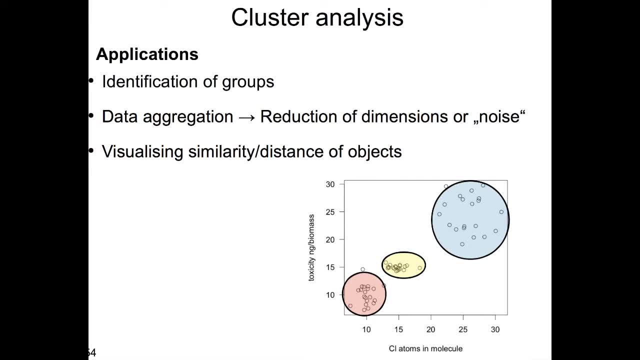 And this reduces the number of groups, And this reduces the number of groups And this reduces the number of groups. Thus the multidimensionality. In addition, it is a technique ch to visualize the similarity and distance of objects. We will later see how we can use a dendrogram to visualize the cluster solution. 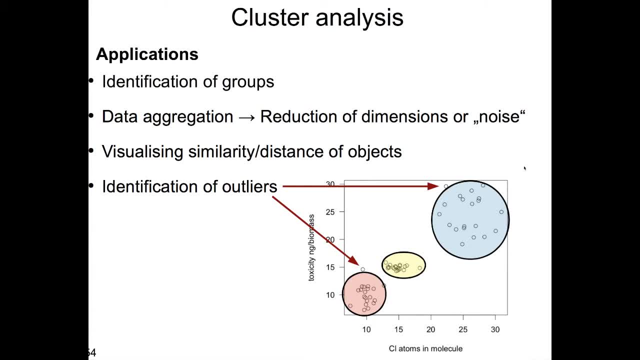 Finally, we can identify outliers. These are points that do not belong to one of the groups. Finally, we can identify outliers can be considered as outliers. they might form individual clusters in a cluster analysis or be merged very late to the clusters that are already existing. 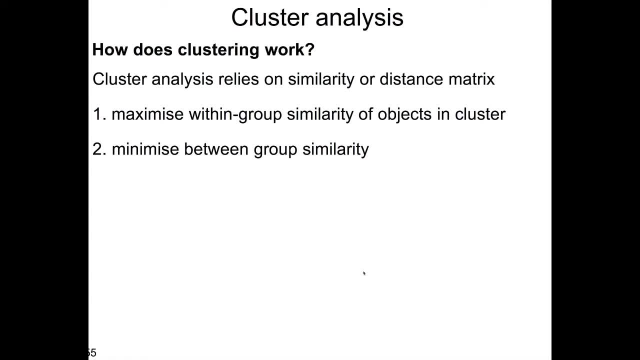 So how does cluster analysis work? It first of all relies on similarity or distance matrix. we have already encountered distance and similarity measures in the previous part of the course, and the aim is always to maximize within group similarity of objects in the cluster and to minimize between group similarity. 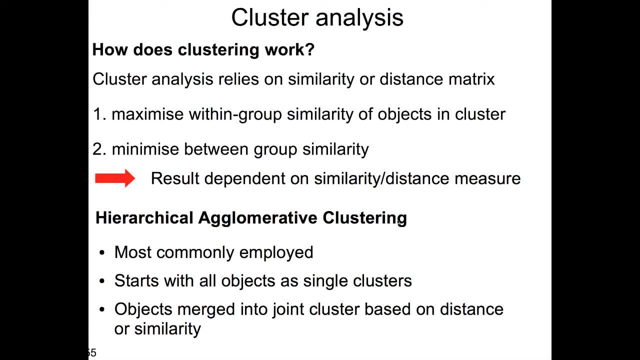 The result is therefore dependent on similarity and distance measure that has been chosen, and there are different types of clustering. The first or most widely employed version is the hierarchical-acclomerative clustering. We will later meet a technique that is non-hierarchical. That means that all clusters are formed on the same hierarchical level and on the other. 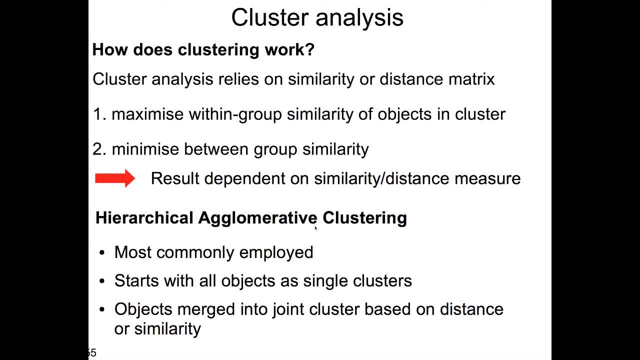 hand, the opposite of the hierarchical-acclomerative would be decisive, which would mean that we start with all objects in one large cluster and break this cluster into groups, while the hierarchical-acclomerative means we start with all objects as single clusters and merge. 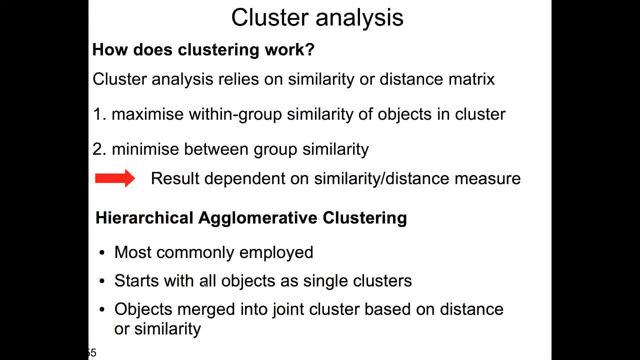 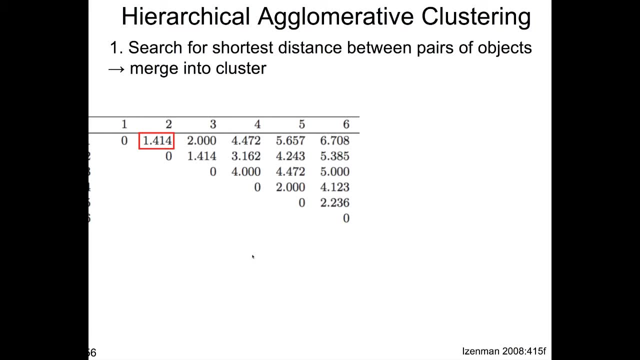 them during the clustering process. The merging is based on the distance or similarity between the objects. What does this mean? How does this work? Let's look for an example. Let's say we have six sites in which we have observed some organisms or some environmental. 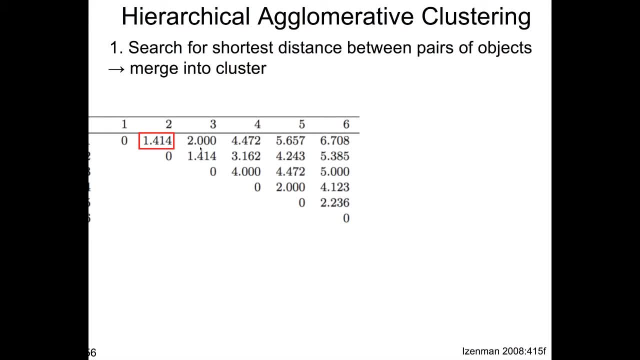 variables and we have calculated a distance matrix. I don't go into details of calculation of distance matrices. We have already done this in previous parts of this course. We have already done this in previous parts of this course. We have already done this in previous parts of this course. 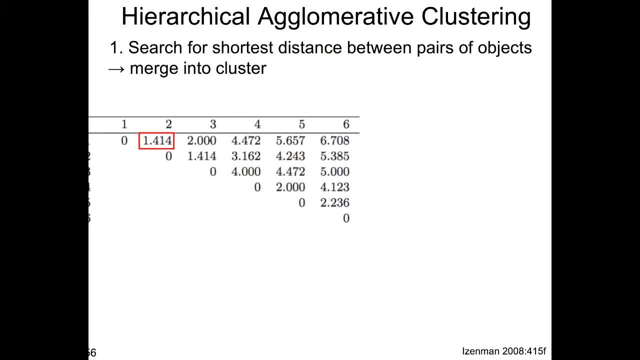 And then we look at the paired distances between objects, between sites. in this case We see that site 1 has the shortest distance to site 2.. Site 2 and 3 would also have a similarly short distance, but we now focus on site 1 and 2.. 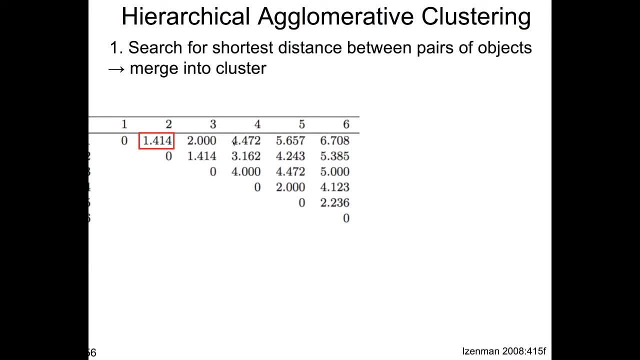 All other distances between sites are larger. All other distances between sites are larger. And then we aside two object at a time. we first merge site 2 and site 1 into a cluster, cried, adequately into one object, And we have now 5 objects: site 3, and side 2.. 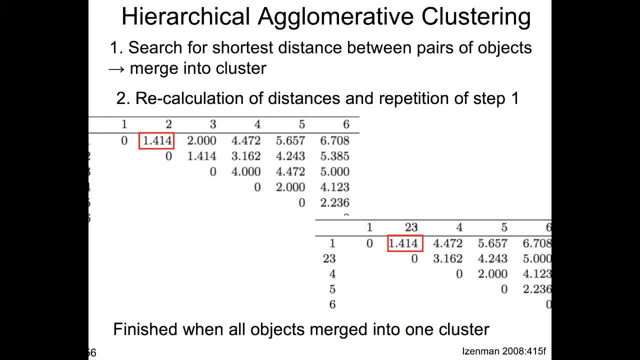 We have object 1 and type 1.. we have the cluster and subcluster for the objects 2 and 3, and now we recalculate the distances with the other objects, That is, we want the goals добавMonitorList. So for site 1, with the cluster 2, 3, we see now that the distance is 1.4. 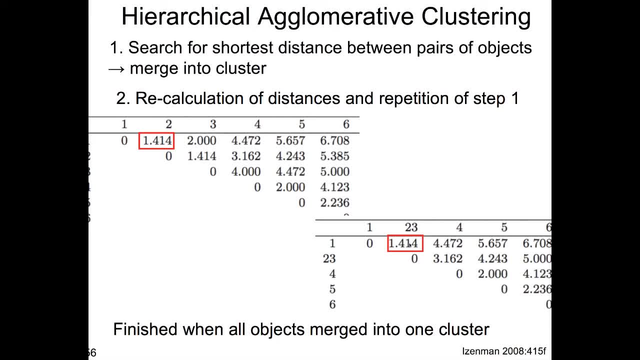 And why this is 1.4, we will learn later on during this session. And we have now distances between the merged site, between the cluster and the other sites. It's not the individual distance anymore And clustering finishes when all objects are merged into one cluster. 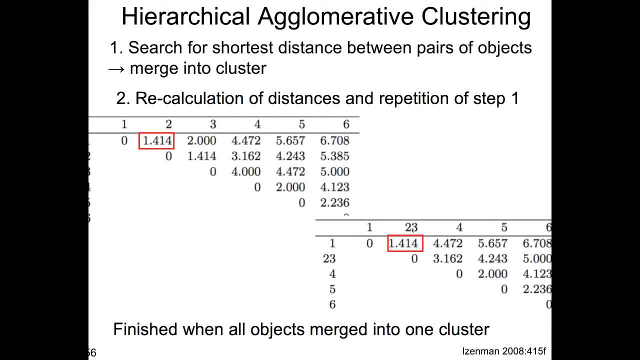 So in the next step we would merge the cluster 2, 3 with the site or object 1.. And then have a cluster 1,, 2,, 3 and recalculate the distances to the sites 4,, 5 and 6.. 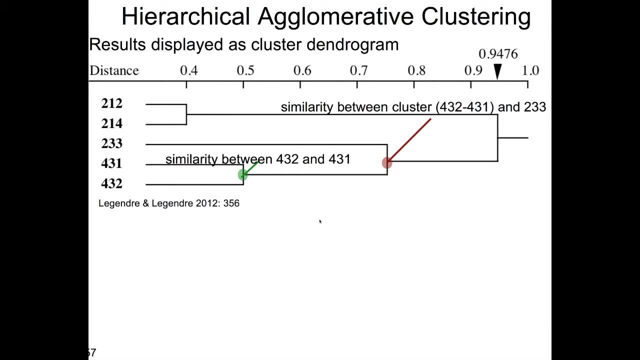 Then we can display the distance. We have the data in a so-called cluster dendrogram. On the cluster dendrogram you have a distance that is displayed along the x-axis, And the further you go along the axis the larger is the distance, And we see that at a relatively short distance here. in this case the two objects 212 and 214 are merged. 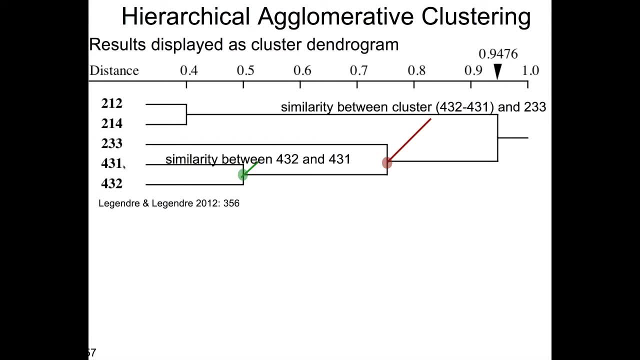 And then the objects 431 and 432 are merged And at this point, at the distance of 0.75 approximately, we merge the cluster 431 and 432 with the object 233.. So what we have here as a quantitative interpretation Is that this is gives you this measure. distance measure gives you the similarity between the cluster and 233.. 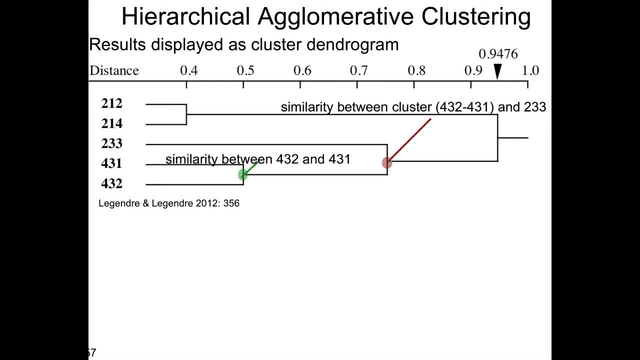 It's not the similarity between 233 and each of 431 and 432.. So that's important to understand. You always interpret the relationship of merged objects of the cluster with the individual sites. in this case, When you have these merging process, This is a little bit similar to the interpretation of a phylogenetic tree. 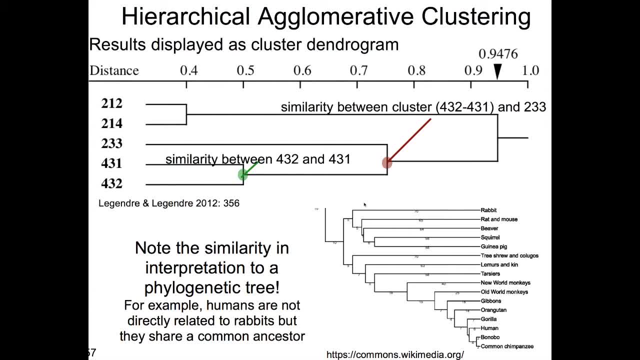 Phylogenetic tree. apart from the fact that the phylogenetic tree is read the other way around, You start on the right side and you can read here at which time there was a common ancestor, For example, between the squirrel and the guinea pig. 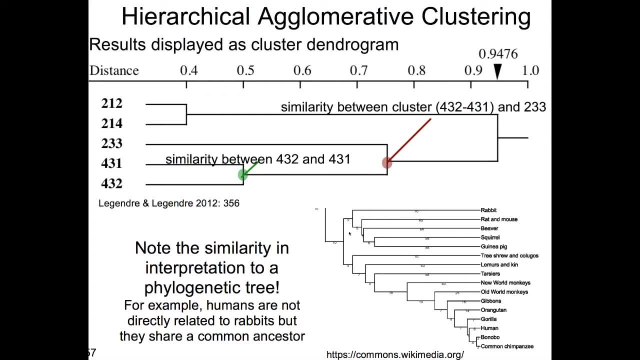 And if you go further, move further back in time, you reach a point where, for example, there were common ancestors of the rabbits And of other organism of another lineage that led to red mouse, beaver and so on. What it doesn't mean is exactly that the rabbit and the squirrel had one ancestor. 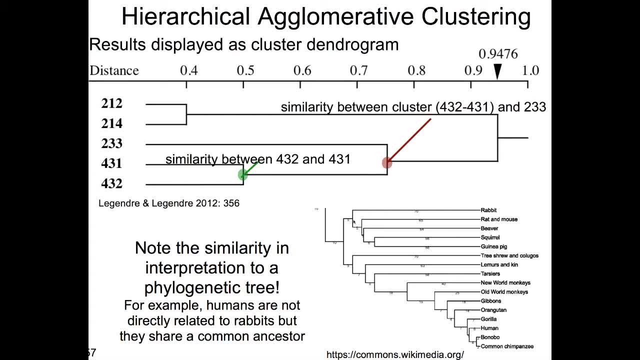 And so on. That was a mixture of them, means only that the mixture of all of these, of all the ancestor of all of these here, had a joint ancestor with the rabbit, And the same holds for humans and monkeys. on this side You have primates, new world monkeys, old world monkeys, lemurs, and so on. 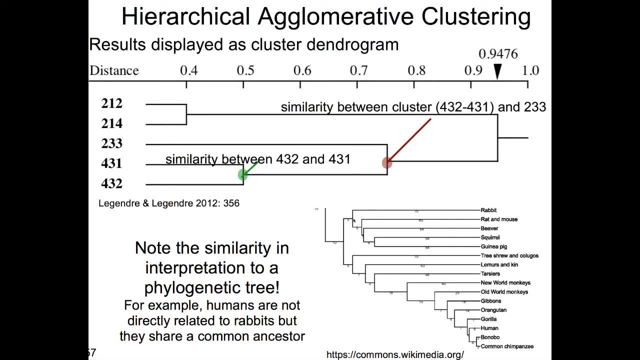 And all these share an ancestor with rabbits. But if you would look at this point And look at the ancestor when there was a split in the lineages, you wouldn't interpret that there has been an animal that was a mixture of a rabbit and a human. 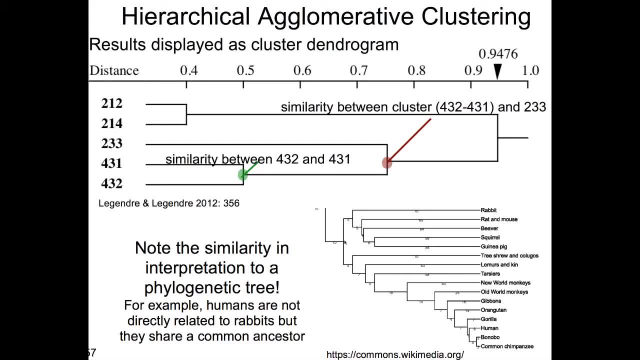 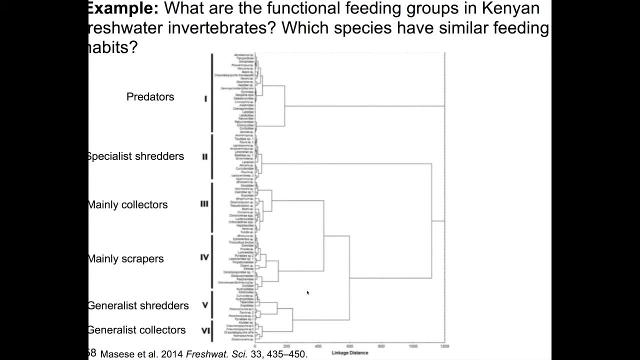 But they just share a common ancestor over several lineages. Let's look at an example. Let's look at an example. where can such an analyzer Be useful? This is an example from invertebrate monitoring in Kenya, And the question was: what are the functional feeding groups in freshwater invertebrates? 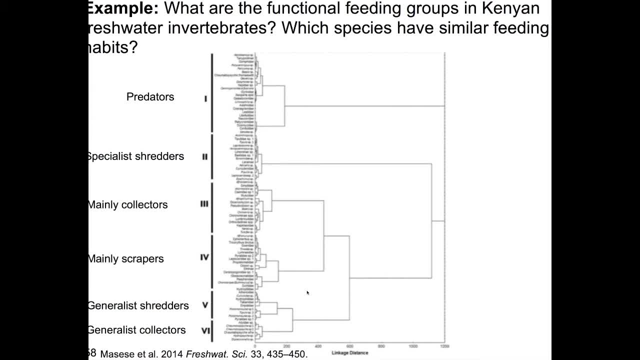 So food webs can give important information on the ecological status of sites, of network relationships of organisms, And such information is therefore useful. So what was done in this study Is that they analyzed the gut contents of the different organisms And then clustered the gut contents for this individual taxa. 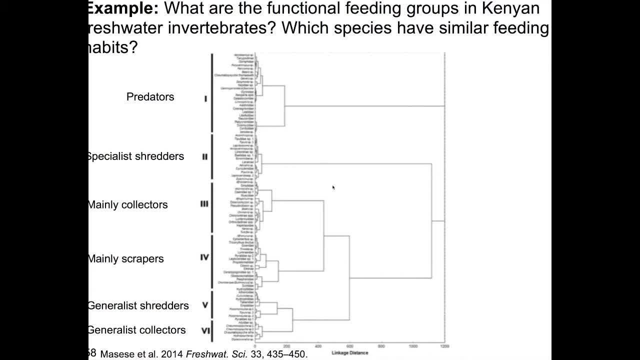 And therefore merged organisms that have a similar gut content. So you see here the cluster solution And what is clearly formed is one group here. So you have relatively small distances For the merging process of the individual objects to clusters, And then you have a very large distance to the next clusters that you see here. 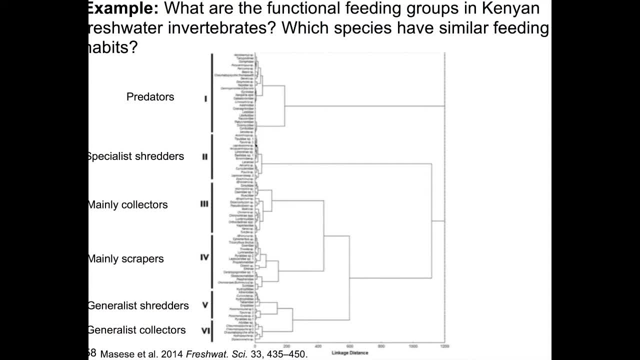 The same you have here. These are rather specialist shredders. These are mainly collector species based on the gut content And so on. You see that scrapers and collectors are relatively similar as well, At least more similar than generalist shredders. 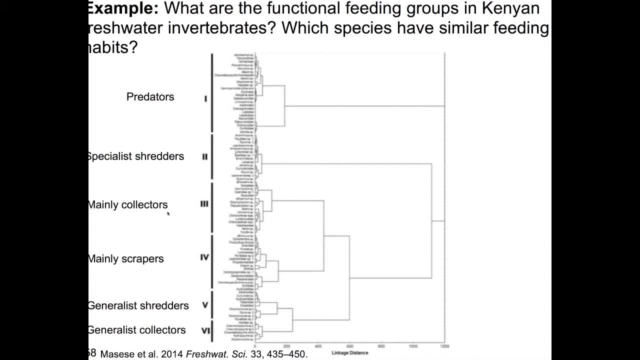 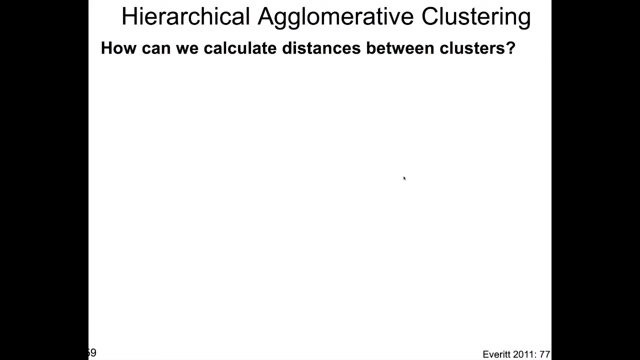 And that means they probably feed primarily or primarily, act as collector, But can also be scraper and vice versa. So how can we calculate the distances between clusters? And this is a very important point to understand. That explains why cluster analysis can have very different solutions. 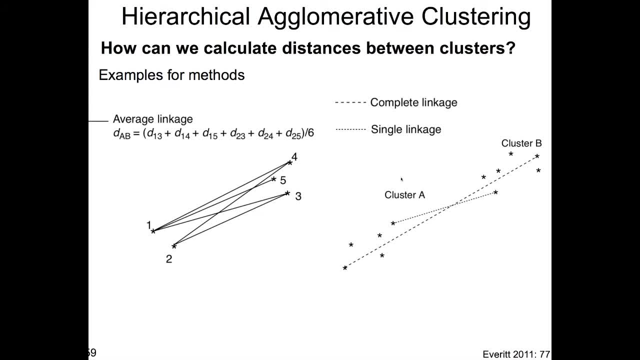 Because when we merge a cluster there are different options. First of all, you could say: well, from our initial points, We just take the average of the distances between the points And calculate the average of all individual distances of all objects in the cluster. But we could also say, well, the distances between two clusters. 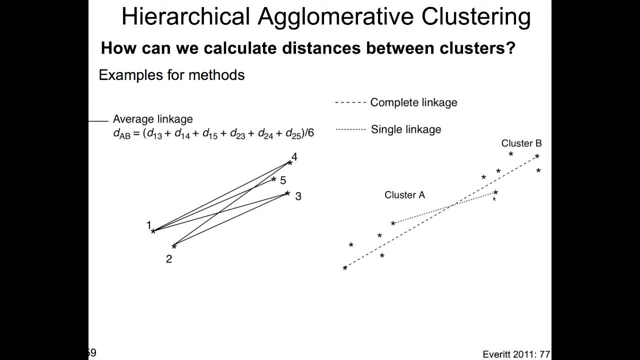 Or between an object and a cluster, Is given by the shortest distance of an individual object, By the minimum distance between the two objects from the different clusters. That's what is shown here And what is called the single linkage. Or we could take the opposite approach. 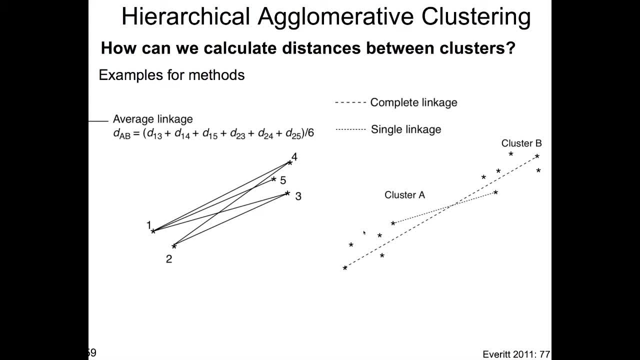 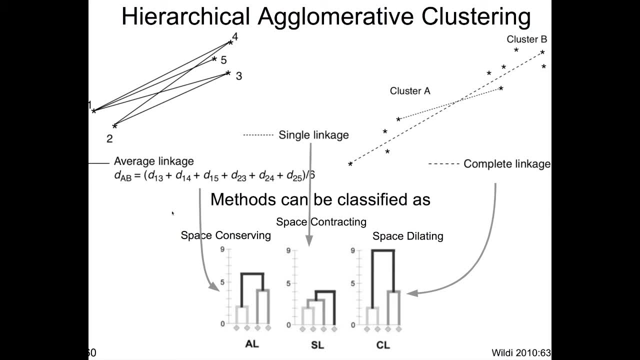 And look at the maximum distance between cluster A and cluster B. Obviously, this leads to very different cluster solutions. We are, on the one hand, We have the average linkage That means the space is conserved. So the distance, the initial distance And the final distance of the cluster solution. 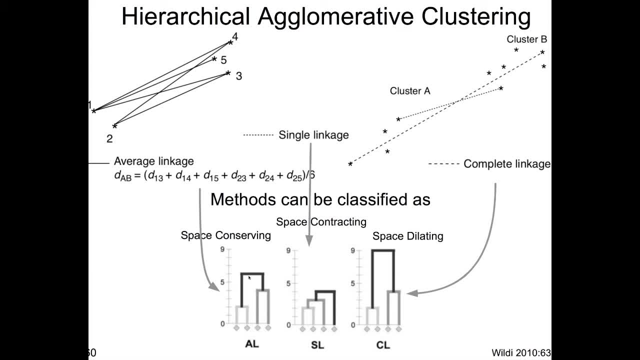 Is relatively similar Because we take the average of the initial distances And therefore it's so called space conserving. We have the single linkage approach That forms clusters based on the minimum distance. That means space is contracted here, So objects move much closer to one another. 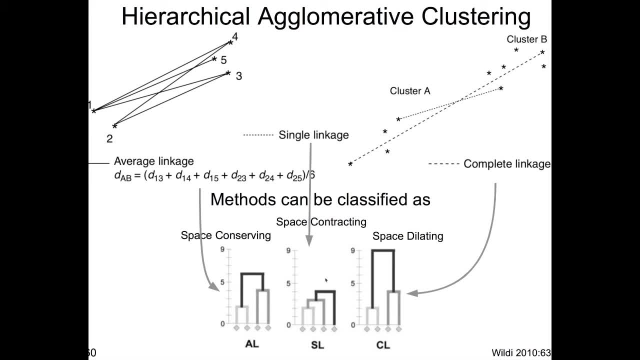 In terms of distance Than they actually are, And we have space dilating methods. That is our approaches. That is the complete linkage approach Where the distances between different clusters are pronounced. So you see here the different pictures For the same data. 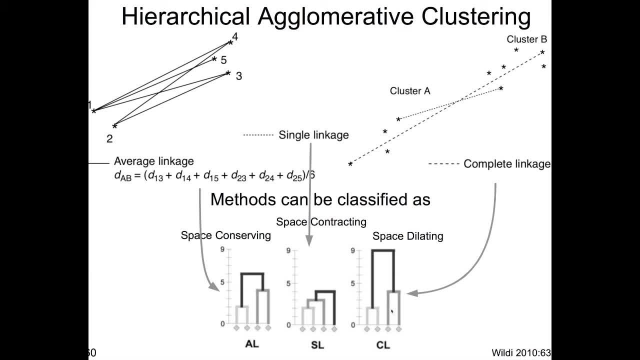 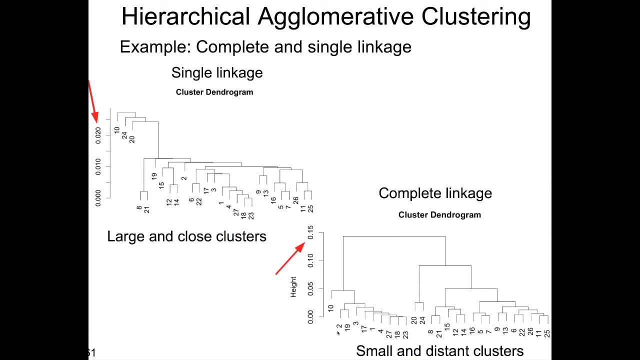 So with the complete linkage We really focus on the differences between clusters Or between the objects in clusters. For the single linkage We focus on similarities. Here is another example for a data set. Really the most extreme cases are contrasted here. 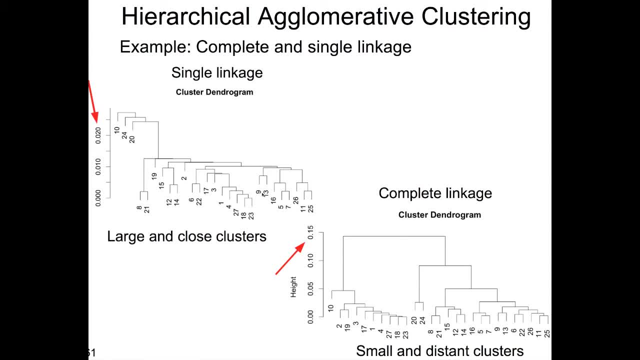 We have on the one hand the single linkage cluster solution. We see that all individual cases from relatively Merge relatively quickly into one cluster. And see here: this is distance. It's called height in R. in the graph, Distance is 0.02.. 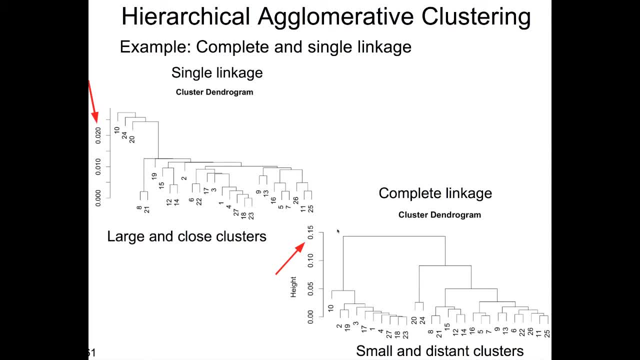 Whereas for the complete linkage, Where we focus on differences, We can see that the distance are much larger- It's about tenfold larger- And we can see that the differences Distances between individual objects and clusters Are higher. We can also see that the clustering structure 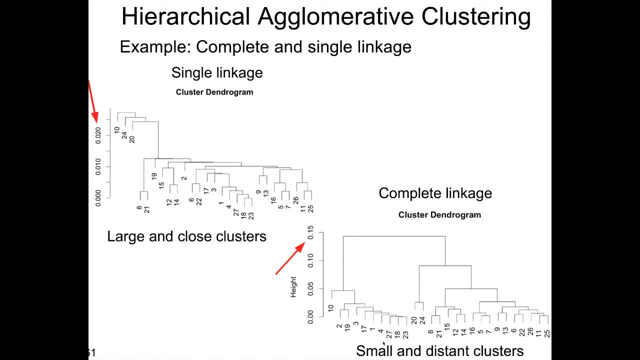 Looks very different. here We obtain small and distant clusters, So we could interpret this That we have perhaps one cluster here, One cluster here And one cluster here, But we have large and very close clusters here, So the structure is relatively different. 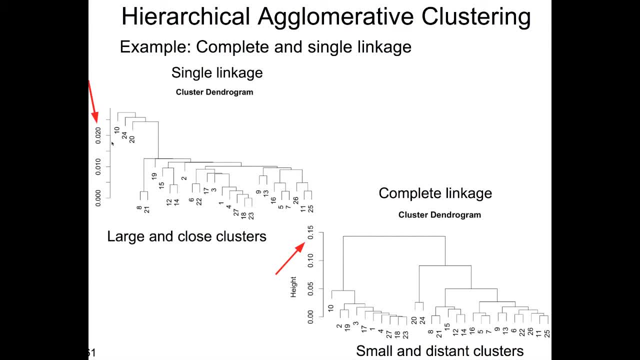 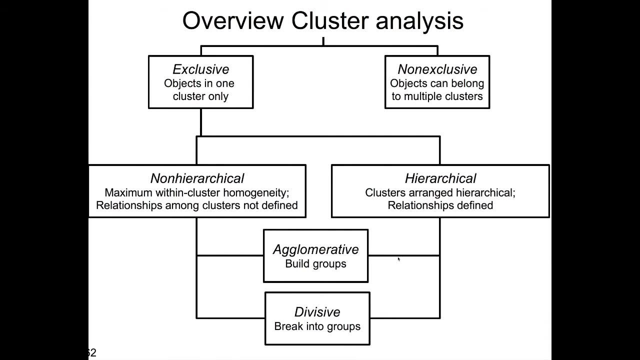 And we would interpret these three as outliers, perhaps, And the other objects belonging into one large cluster, And a different interpretation Would hold for this complete linkage approach. So there are many more options in cluster analysis. You can have exclusive clustering And non-exclusive. 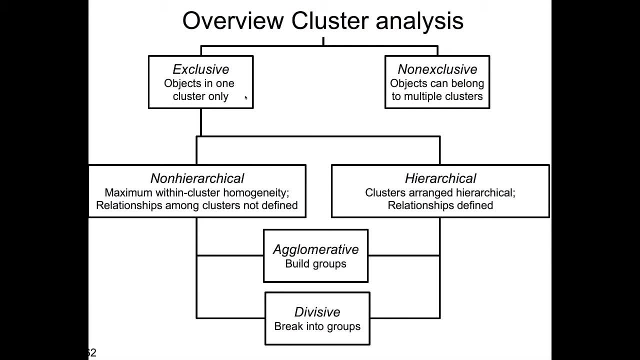 Exclusive means that objects are just put in one cluster. That's something that we have followed so far. And then we took the approach for hierarchical clustering. It means clusters are arranged, hierarchical Relationships are defined. That is something that we have seen so far. 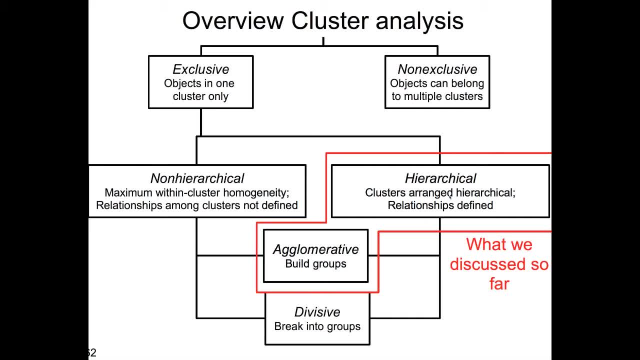 So we have these dendrograms, These trees that emerge from the cluster solution And we can also, We will also look at non-hierarchical clustering. That means We have maximum within cluster homogeneity But that there are no relationships Or defined relationships among the clusters. 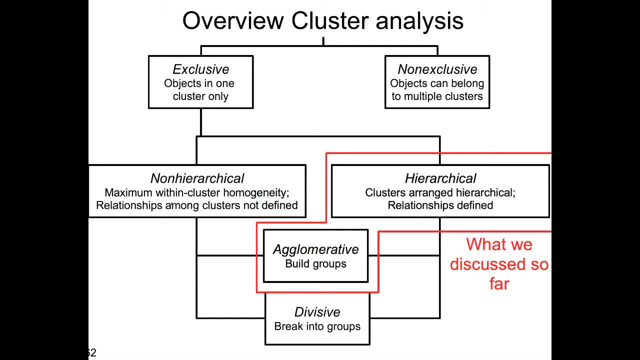 And that means we don't have a cluster dendrogram Or a tree Like we have seen before. The Acclomerative clustering means We build groups. The divisive would be: We start with one cluster And break groups. I've already mentioned this. 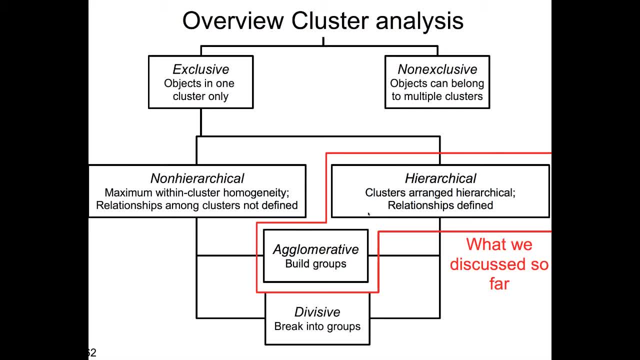 And this is the approach we mainly- will look at Hierarchical acclomerative clustering And afterwards, Non-hierarchical Acclomerative clustering. Non-exclusive clustering would mean That object has a membership value And can be assigned to different clusters. 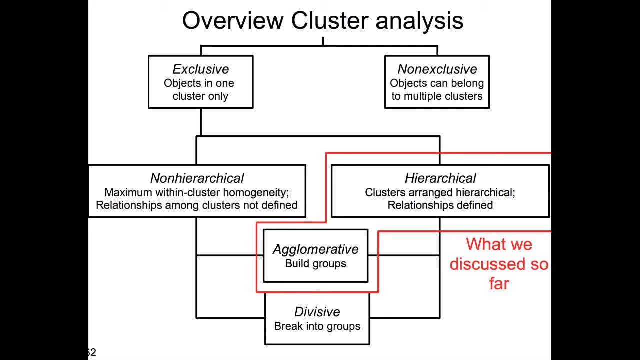 You can have overlapping and continuous clusters. This Different approaches Or can be Looked up in the Everett 2011 book That is very useful for clustering, And Look for the topic of fussy based clustering And overlapping clustering. 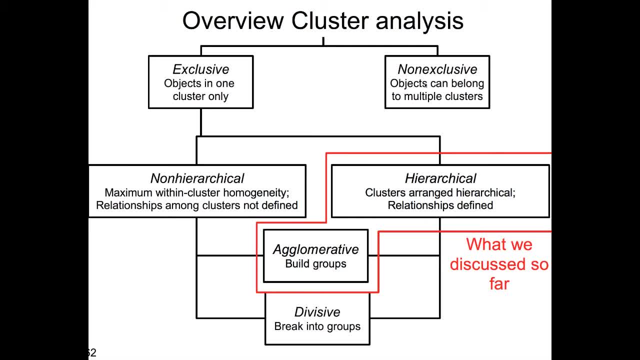 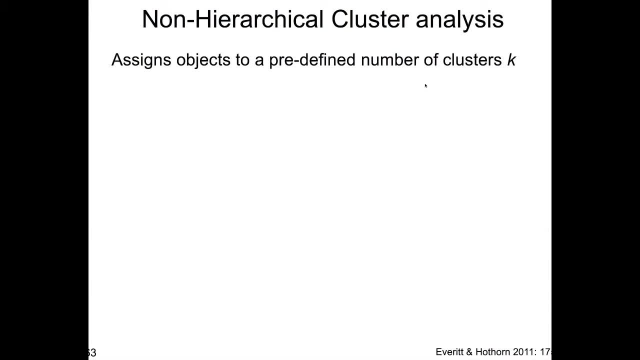 In R, The function or the package that you would use Is called: Is the package cluster And the function. funny. Now we move on to non-hierarchical cluster analysis. In this analysis, We have Assigned objects To a predefined number of clusters. 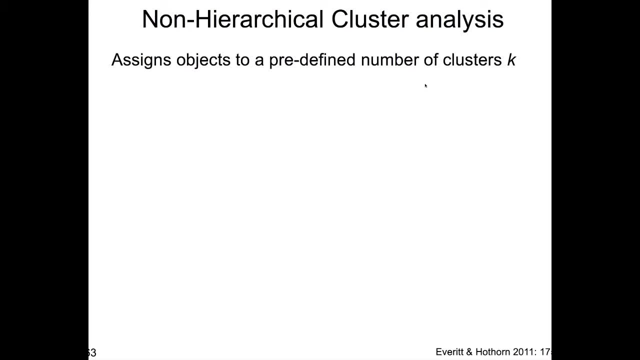 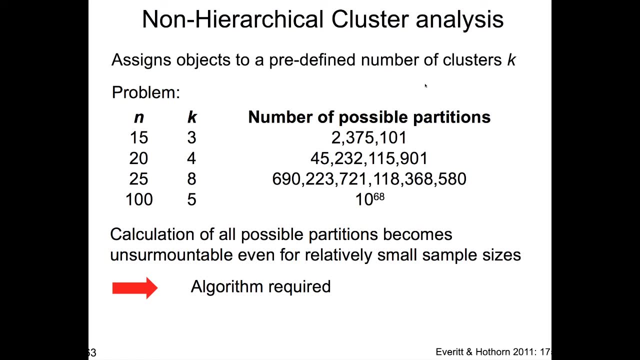 K. So we need to define before Whether we want to Have four, Five Or six different clusters. And the problem that comes up here Is The illustrated here. Let's say we want To look for three groups And we have a sample size of 15.. 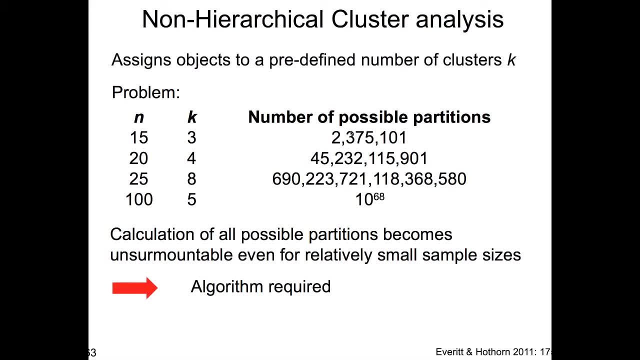 That means That we have all Already Two million possible partitions of the Of the objects between The clusters. in case We look at Identity of the Groups as well, Let's say we have Four groups And have 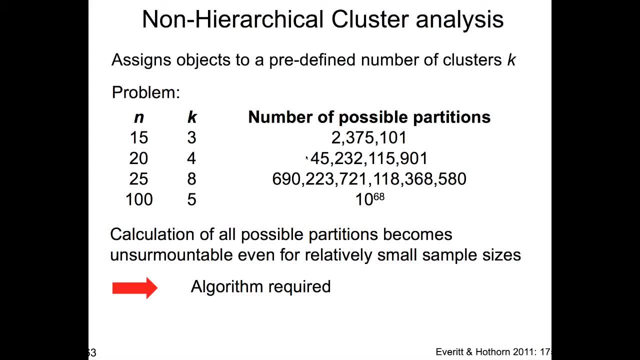 20. Different Samples, Then we are already facing Facing 45 billion options And the problem Gets more or less unsurmountable. And When we have A sample size Of 25. And Eight Different, 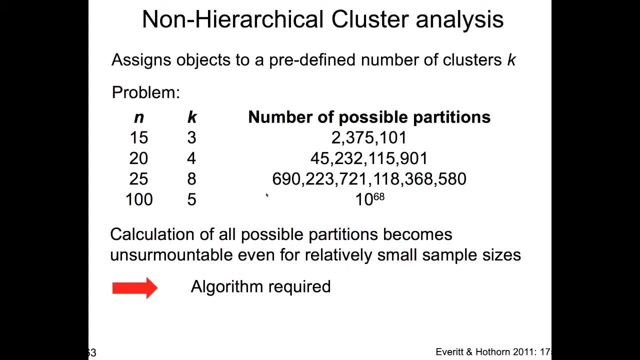 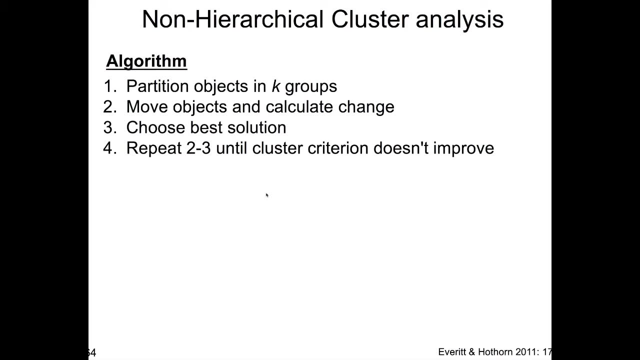 Groups. So Calculating Is Relatively Difficult For All Possible Solutions. So you need some kind of Algorithm. And what Does This Algorithm To Do? The What Does? 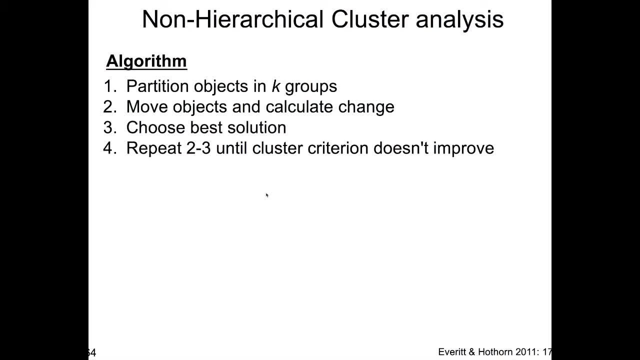 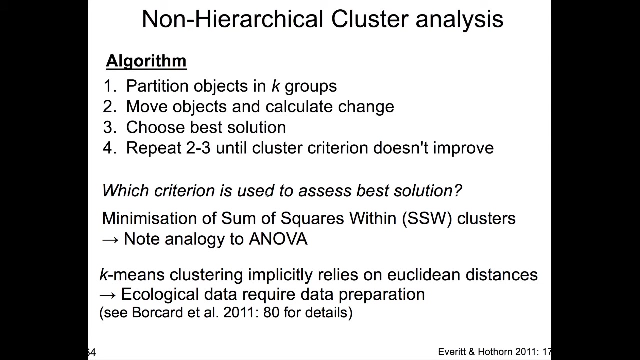 The Algorithm Do, Then It Moves Objects And Calculates The Change And Chooses Afterwards The Best Solution And Repeats The Steps Two To Three Until. 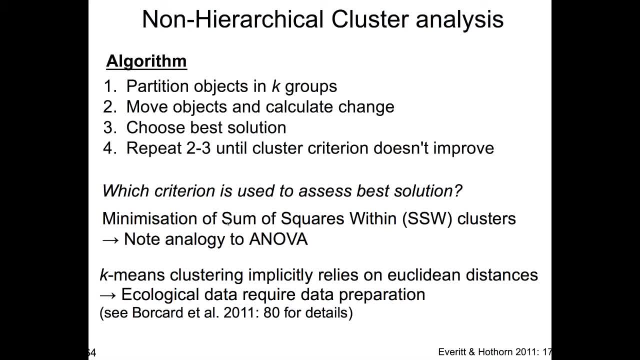 The Cluster Criterion Doesn't Improve. So What Is The? The Cluster Sum Of Squares. And Here You Note The Analogy To An Over An. 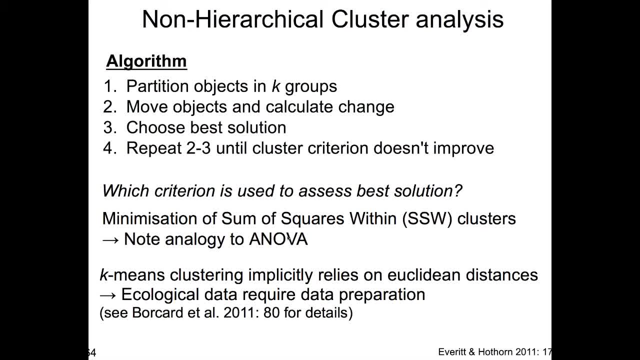 Over In The F Test Is Also The Ratio Of Within Sum Of The Similar Of The Test Statistic That Is Used. It Relies This: 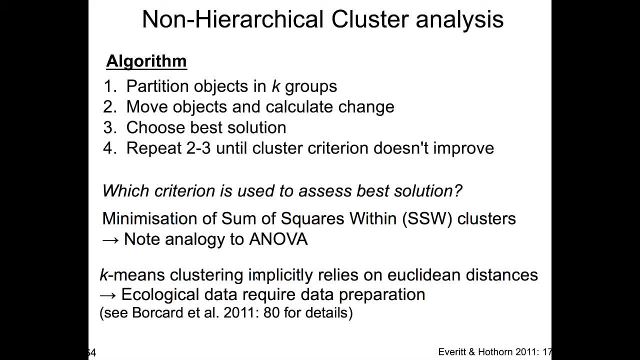 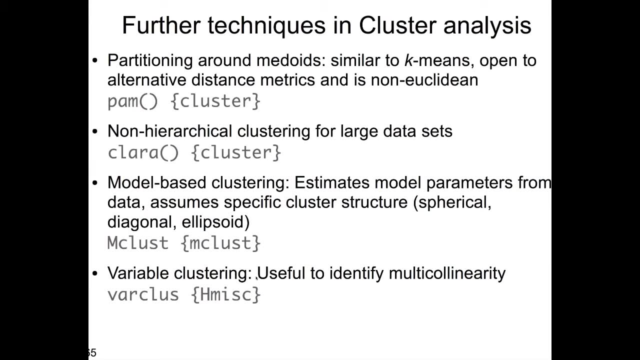 Clustering Says K Means Clustering Implicit Relies On The Euclidean Distance. Again, A Similarity To The An Cluster Analysis Is Partitioning Around Meteorites. 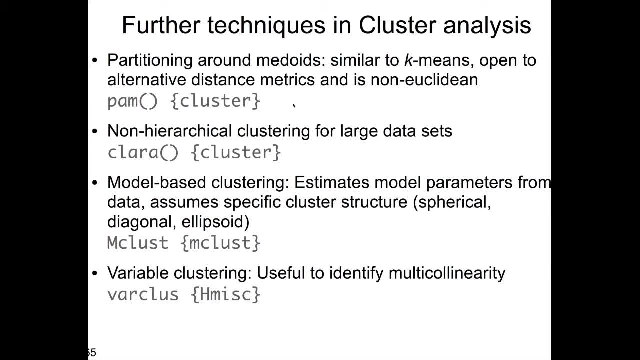 So It's Similar To K Means, But You Can Use Different Distance Metrics And It's Non Euclidean. You Can Have The Non Hierarchical Cluster. 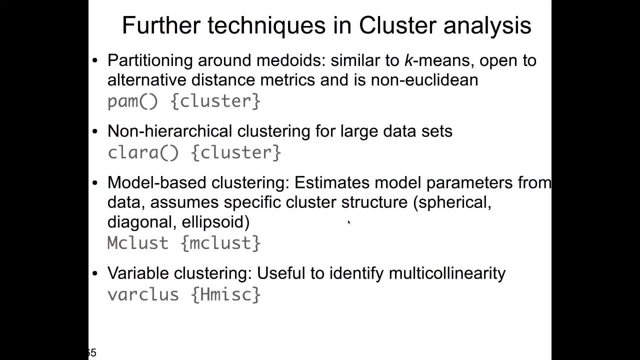 And Assumes A Specific Cluster Structure And Does Hypothesis Testing And You Can Finally Have Variable Clustering, Which Is Really Useful To Identify Multicoloniality. 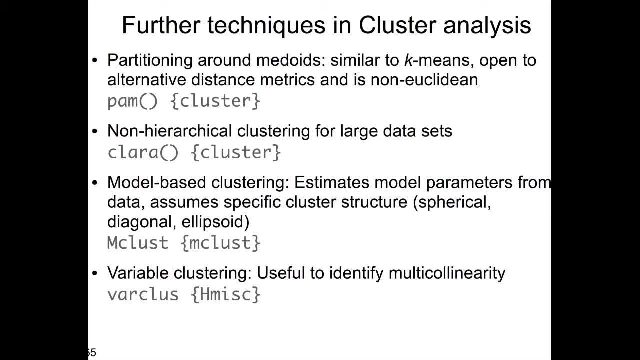 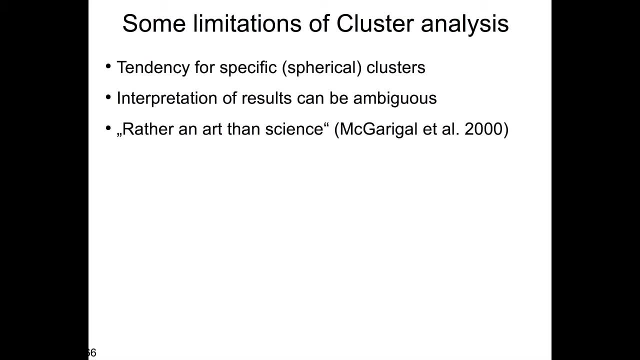 So It Creates A Dendrogram Of Some Limitations Of Cluster Analysis. There Is Clearly A Tendency For Specific Spherical Clusters, Which The Approach 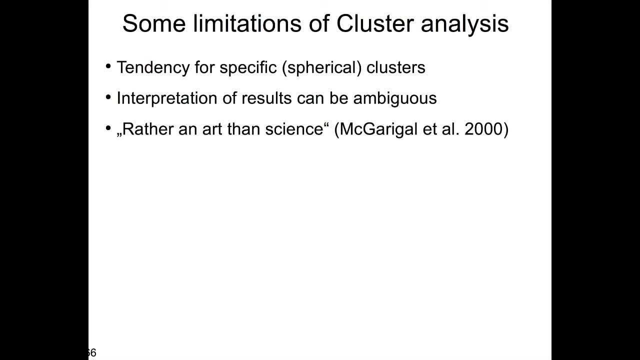 Is Basically Picking Up, You Have Interpretation Of Results. That Can Be An Art Than A Science. Nevertheless, It Represents A Valuable Tool For 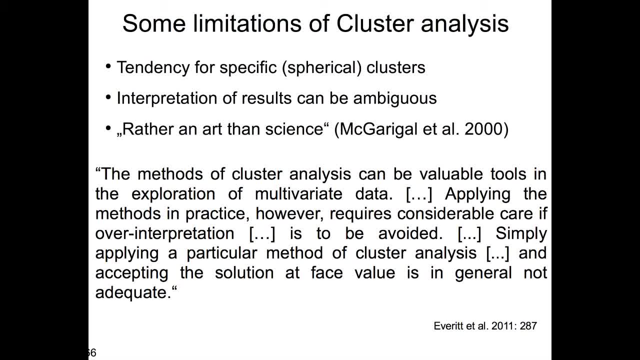 Exploratory Studies And In Different Scientific Fields. So I Want To Finish This Portray Of Cluster Analysis Of Multivariate Data, Applying The Methods In 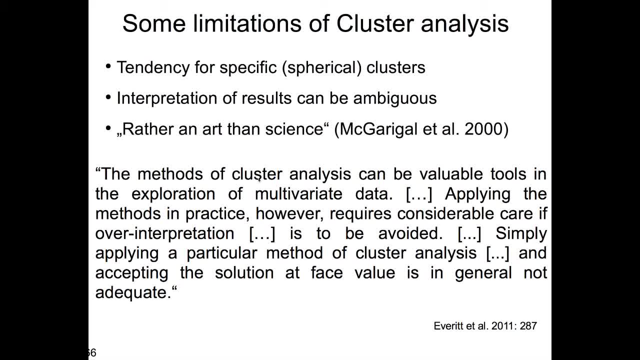 Practice, However, Requires Considerable Care If Over Interpretation Is To Be Avoided. Simply Applying A Particular Method Of Cluster Analysis And Accepting The 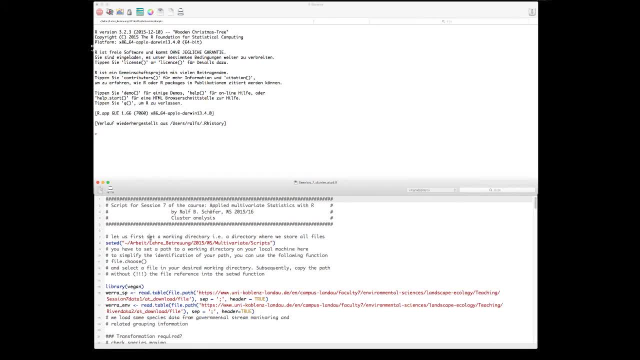 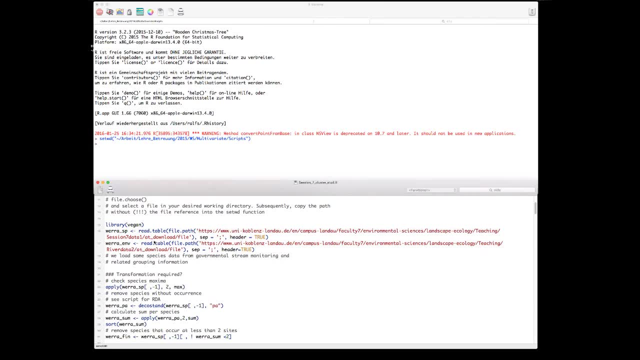 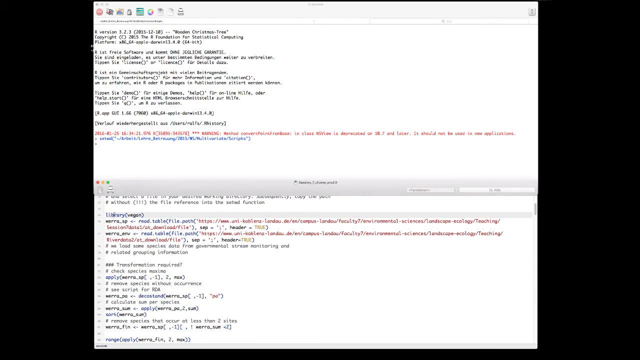 Request And A Service And The One That You Can Open Your Script. We Have The Student Script Here And The First Thing That We Typically 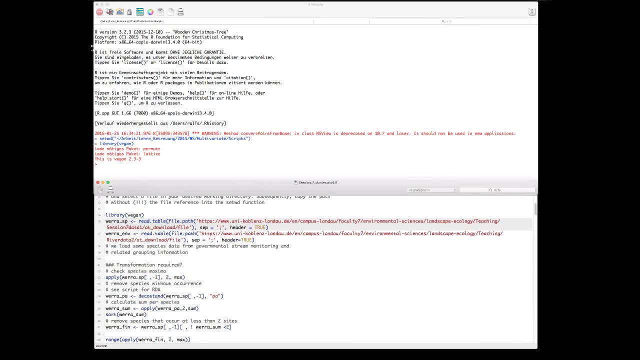 Do Is That Includes Information On Governmental Stream Monitoring, On The One Hand, Species Information That Have Been Found In The Science And, On The 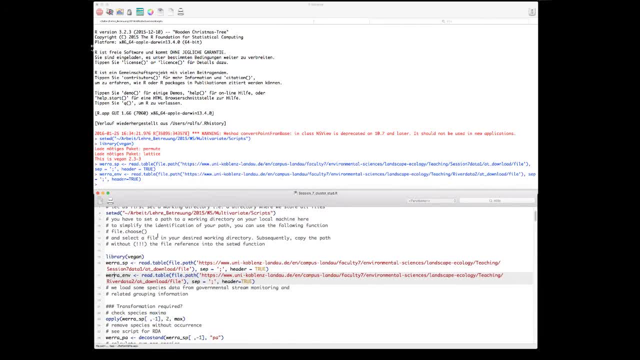 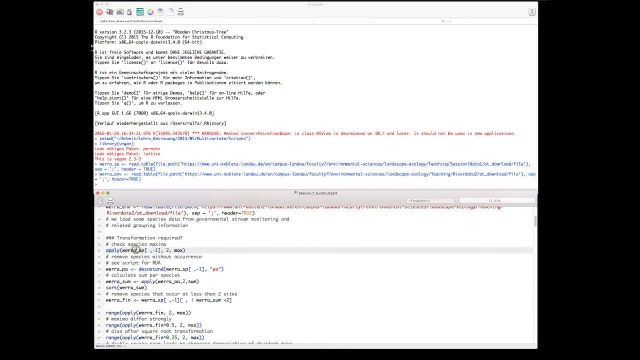 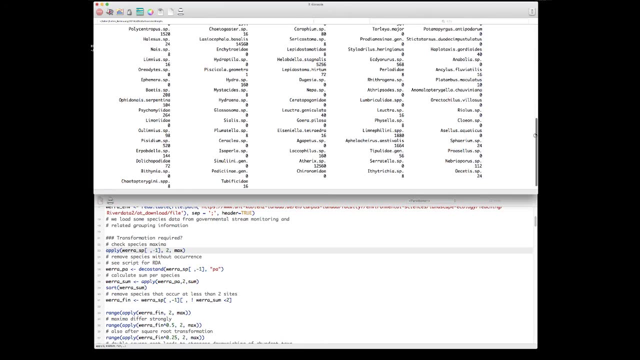 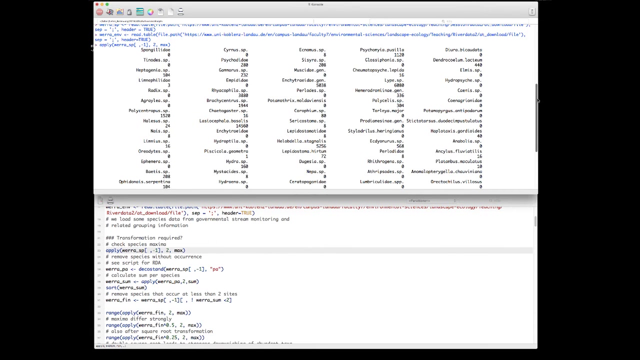 Other Hand, We Have Information, This Grouping Structure, So We First Check For Them When We Work With Species Data. What Are The Species Maximal? 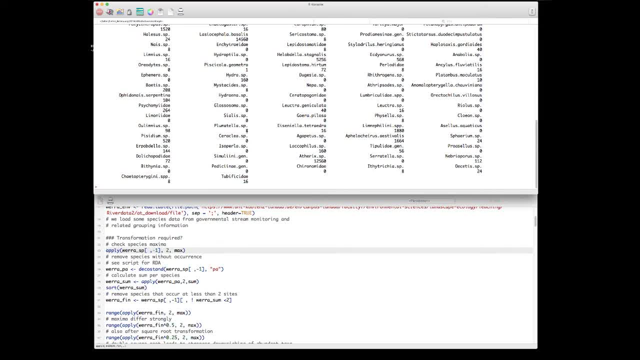 On Where. What We See In An Overview Here For This Is That We Need Some Down Weighing Of Highly Abundant Taxa, Because 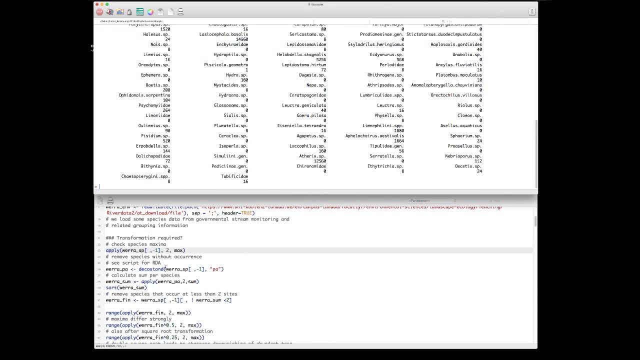 Otherwise, All Distances Will Be Governed By The Highly Abundant Species In Addition. We Want To Remove What We Have Done In The RDA. 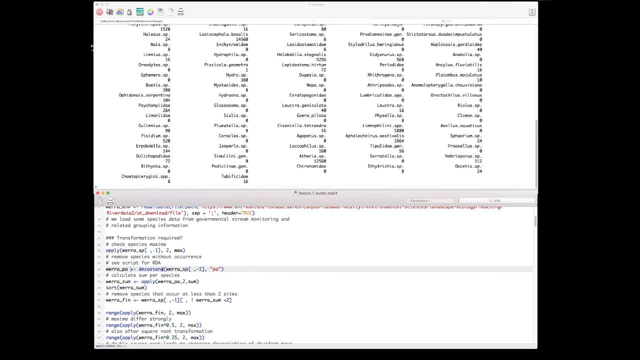 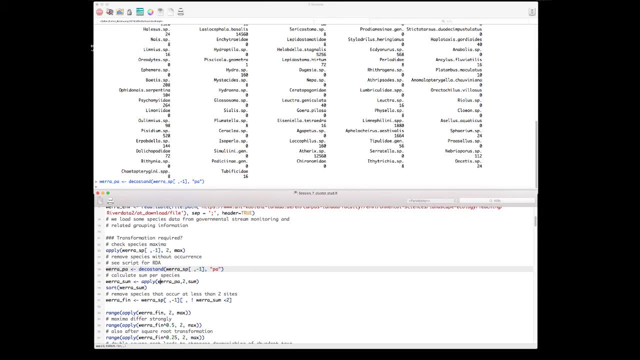 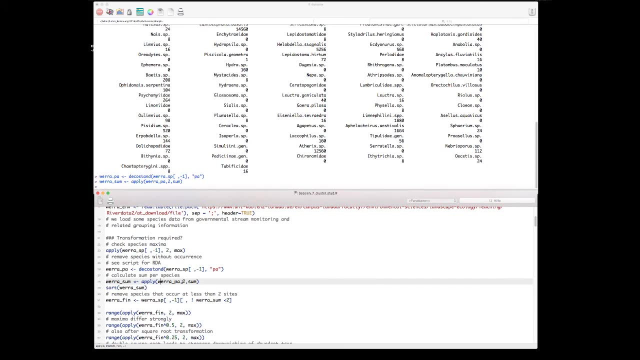 Analysis. Check Out The Script If You Don't Know This Anymore. We First Calculate The Presence Absences For The Data, And Then We See. 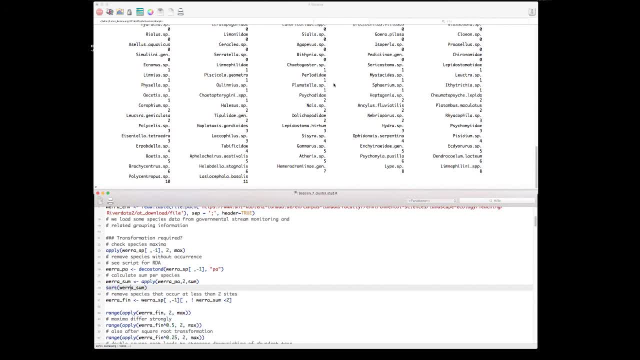 That There Are Many Species That Never Occur In The Data Set And Some That Just Occur In One Of The Sites. Given That, We 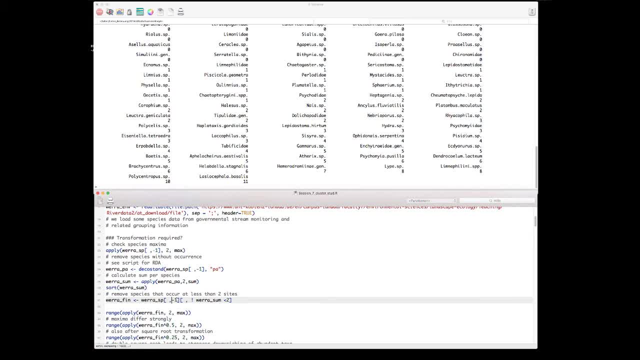 Look For The First Column Of The Data Set. The First Column Gives The Site And We Don't Need This. We Only Want To Have 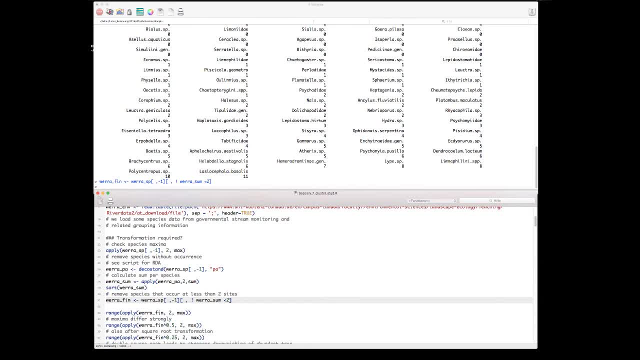 The Pure Species Information For The Data. Then We Apply The Function Maximum To See Again The Differences Between Abundances And Species And We See: 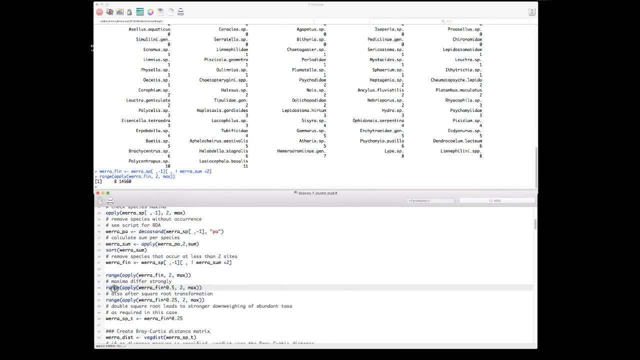 That Still The Range Is From. One Species Has A Maximum And A Magnitude Between The Maxima And The Species, So We Choose For The 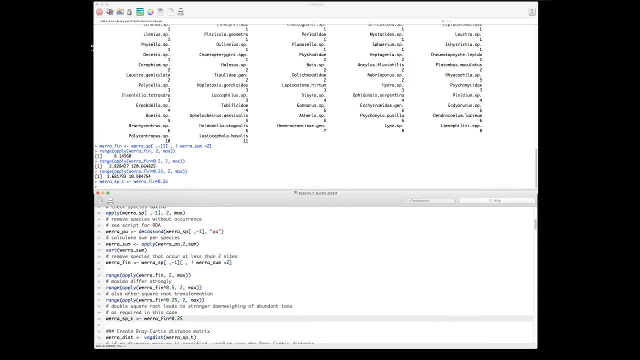 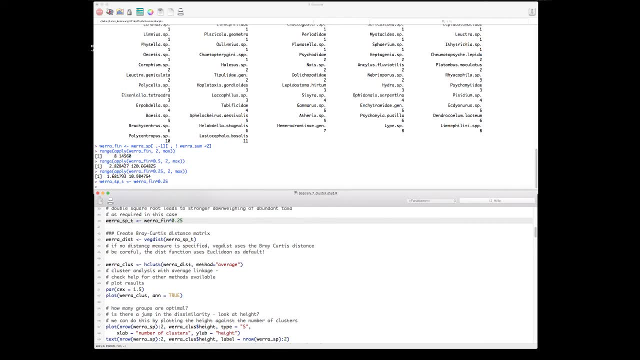 Later Analysis, The Double Square Root Transformation, Which Means That We Have The Maximum Within A Precurtains And This Automatically Applied If You Execute. 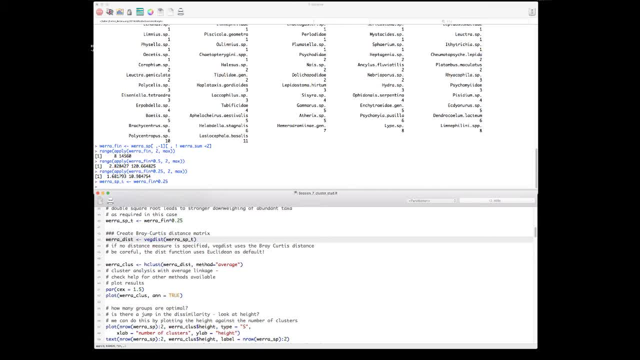 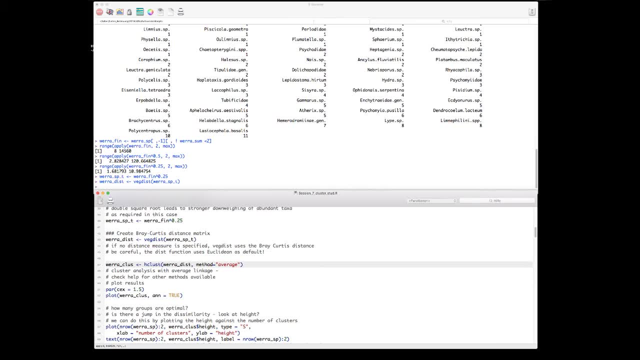 The Vectist Function. However, Be Careful That In The Dist Function There Is Euclidean Distance, The Default Setting, And Now We Run Data Distances. 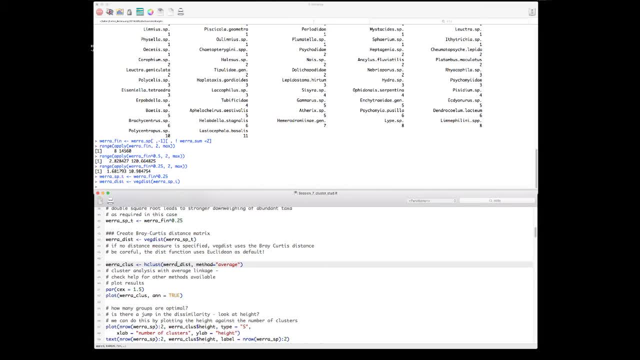 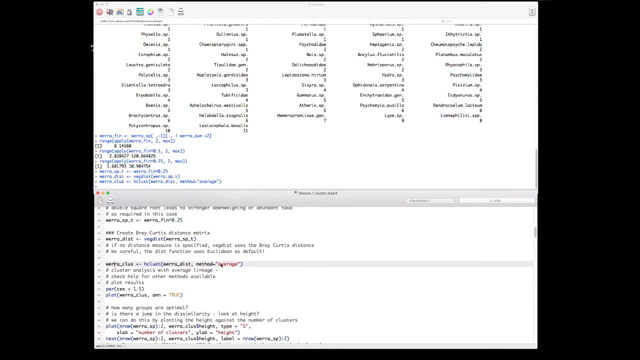 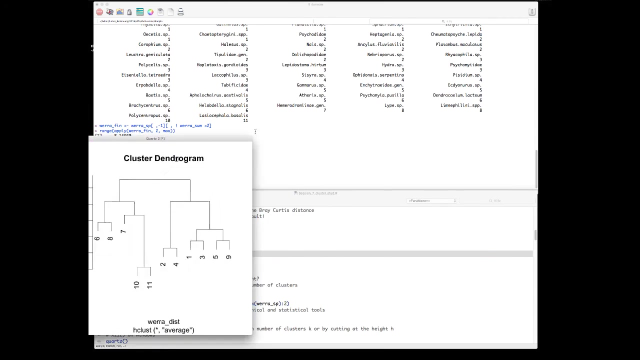 Between The Individual Objects In The Data Distance Matrix And We Select A Clustering Method. Here We Select The Average Method. That Means We Try. 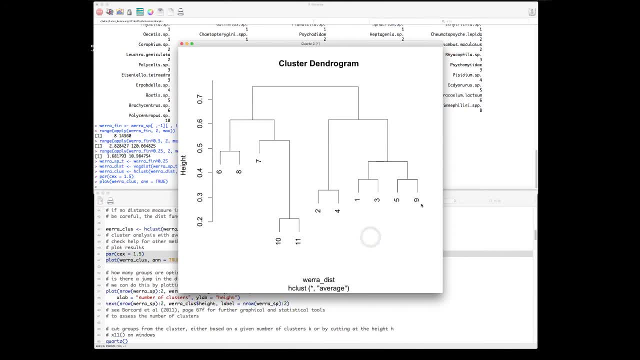 To Conserve The Different Sites From Which The Species Originate, And We Can See That We Have Mostly Two Sites That Are Relatively Similar. 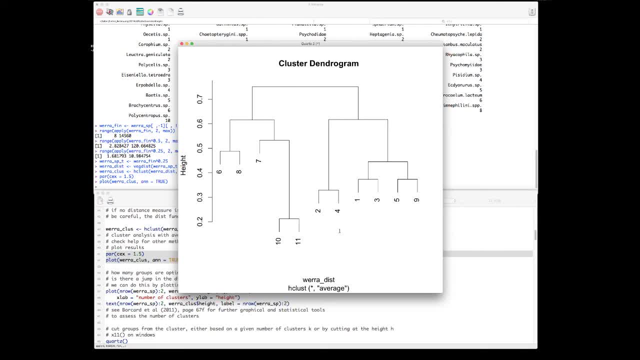 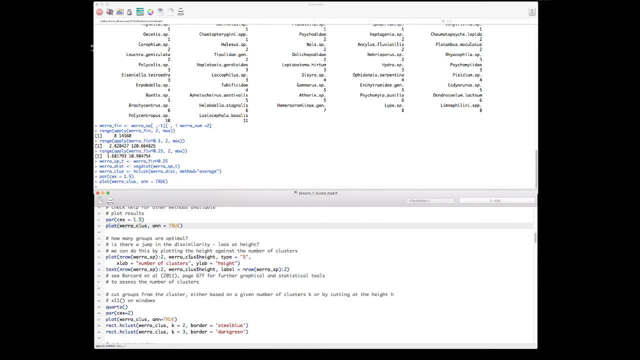 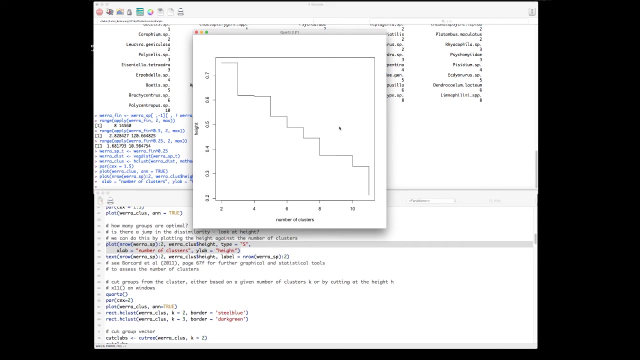 That Are Quickly Merged With Each Other Apart. Now We Have To Ask How Many Groups Are Optimal. Is There A Jump In The Similarity? 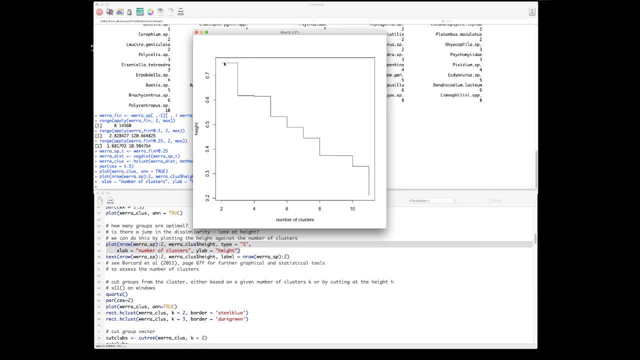 Or Where. What Should We Look At? And We Look Whether We Have Three Clusters, And Then This Continues Until We Have Very Many Clusters. 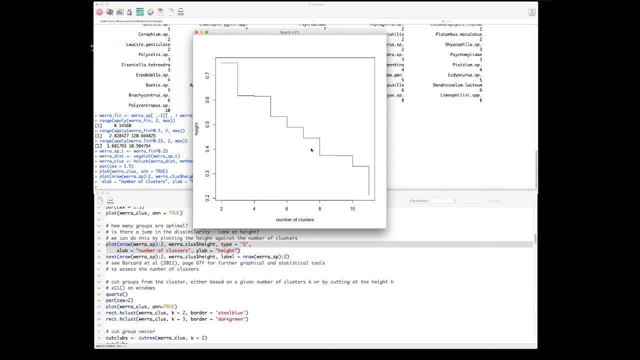 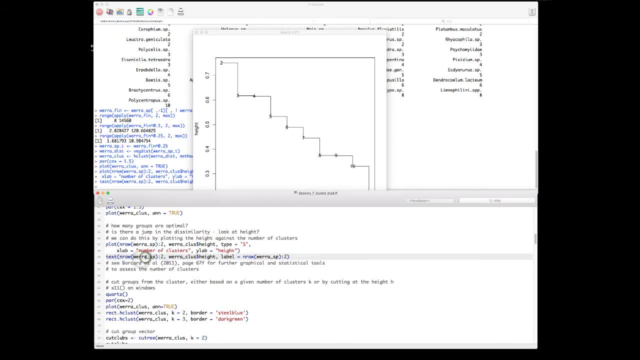 So Perhaps Also There's A Larger Jump In The Beginning From 12. To 11. Clusters And So Different Steps In The Clustering And 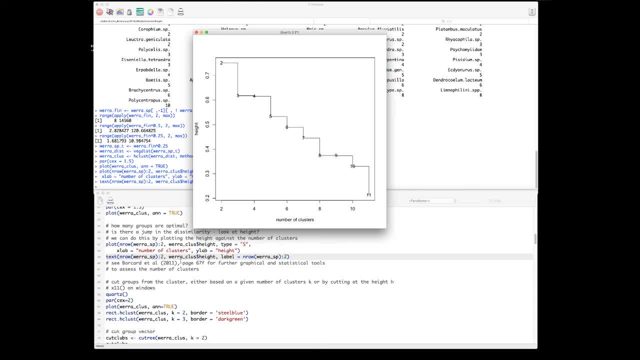 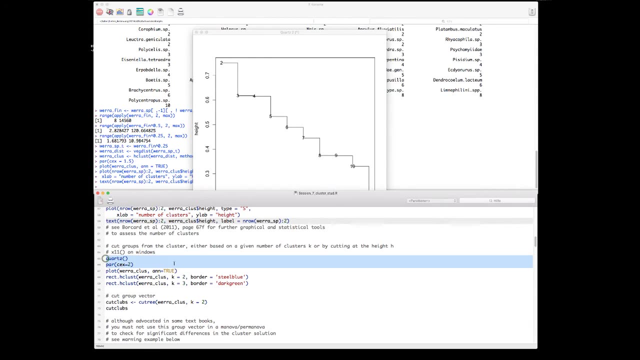 This Plot. There Are Different, Many More Graphical And Statistical Tools To For Deciding How Many Crops Are Optimal. Groups Are Optimal, But 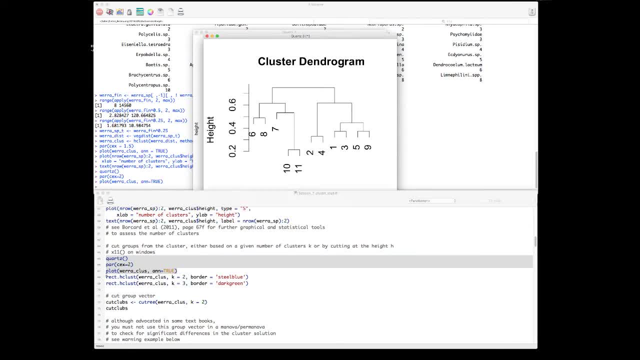 You Use Different Techniques And Different Function. It's Direct H Class Argument, And This Argument Uses The Cluster Solution. You Provide Here How Many Groups. 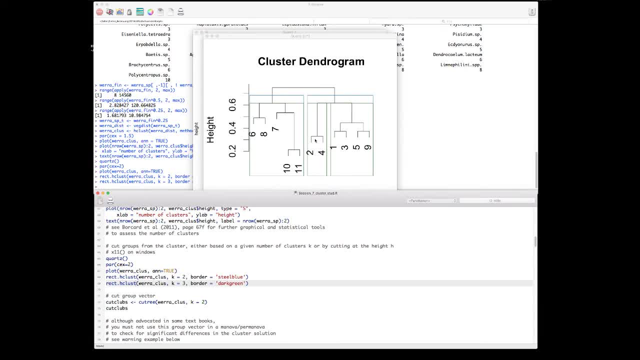 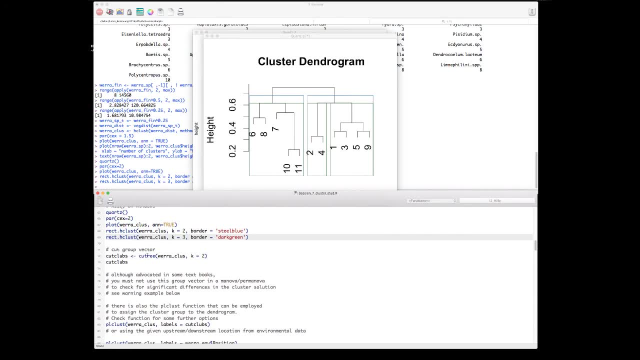 You Find Optimal And Have This Solution- And It's Indicated In The Plot- You Can Also Use This Result Now To Assign Memberships To. 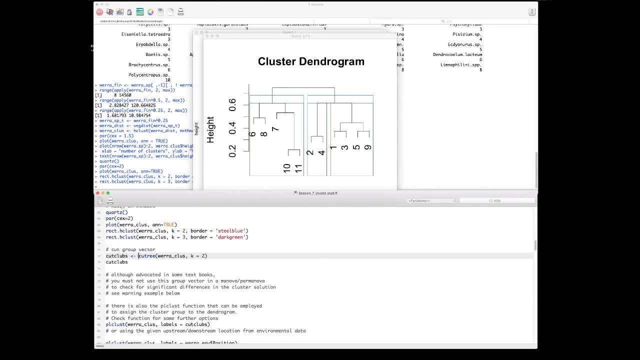 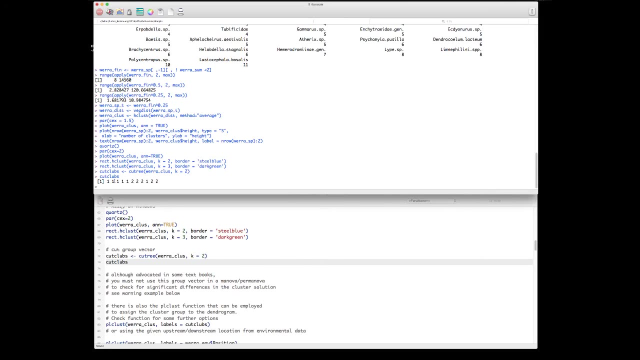 The Individual Data. So With The Cut Tree Function, You See What We See Is. Then We Obtain A Vector That Tells Us To Which Cluster 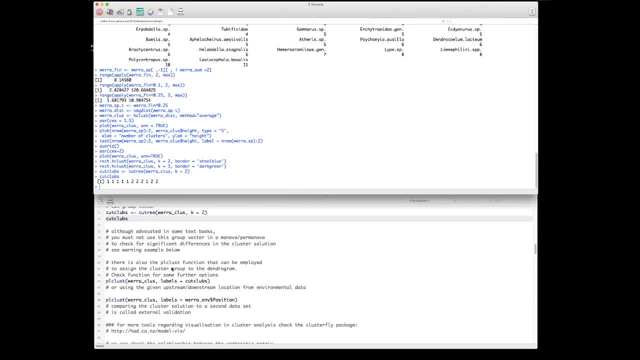 The Individual Objects Belong To. So This Gives You The Grouping Structure, So Such A Data, That Is A Part Of The Data, So For. 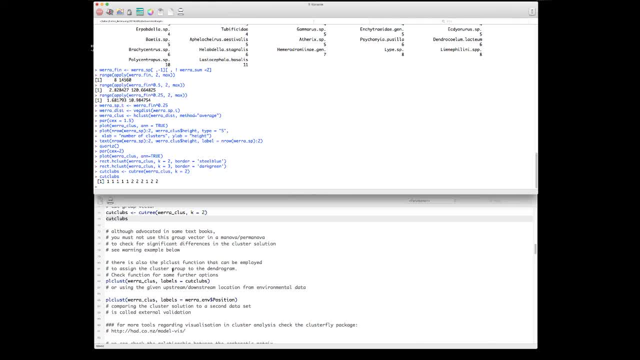 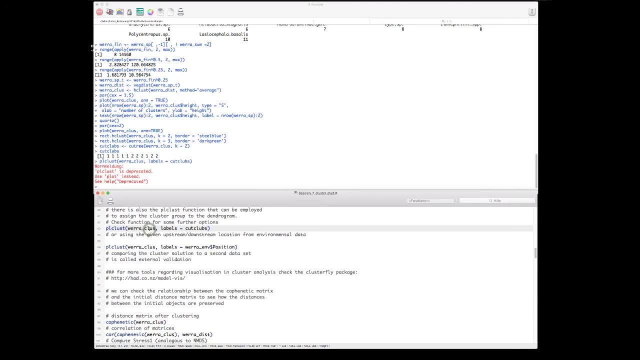 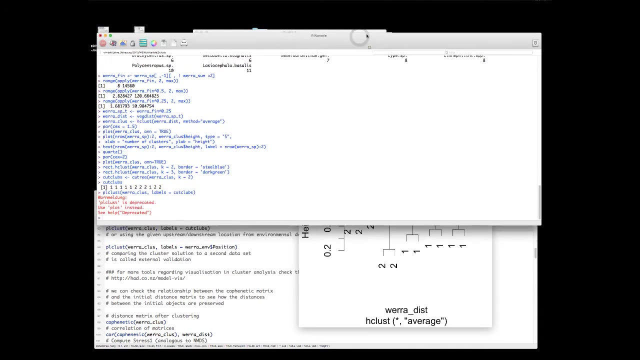 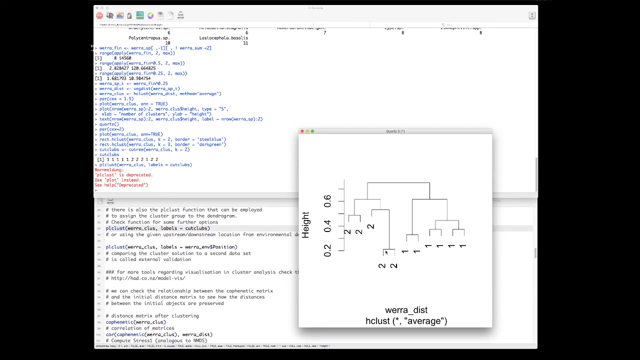 You To Assign Memberships To This Part Of The Data. So This Is A Part Of The Data. So The To Which Cluster And The 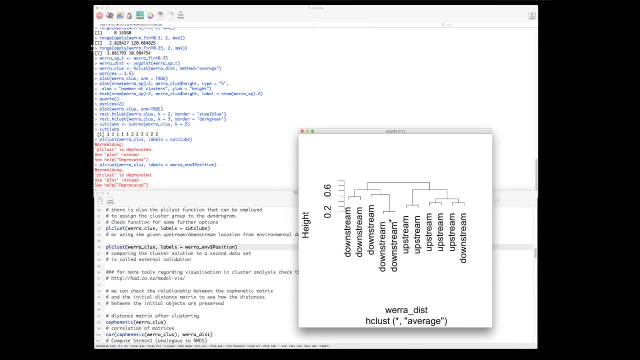 Individual Objects Belong, And You Could Also Use Labels For These Type Of Globs Plots. It Seems There Is A Part Of The Data. 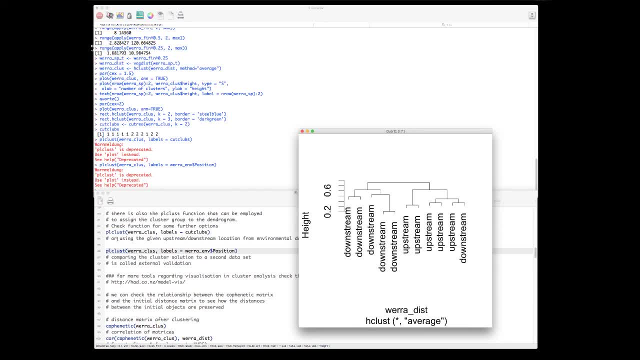 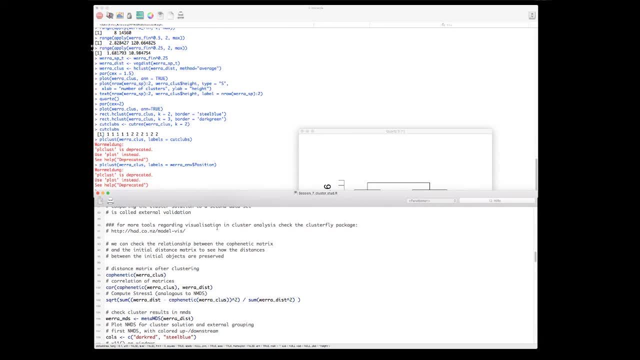 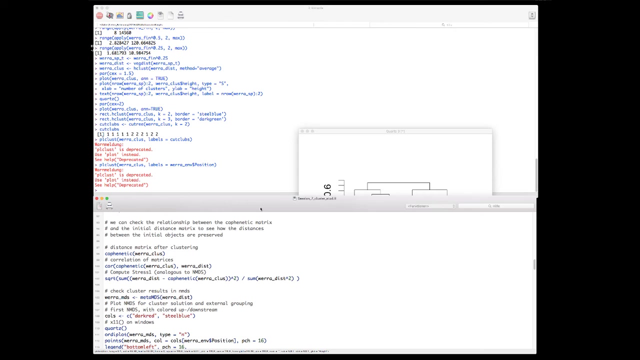 Function. Instead, There Are More Tools, And They Can Be Checked Here On The Website For The Cluster Fly Package. Now Let's Look At The 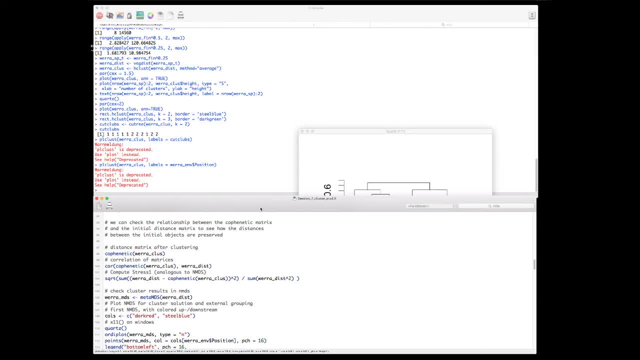 Initial Distances, And The Cluster Solution Is Provided In A So Called Co Phonetic- Co Phonetic Matrix. So What We Can Do Is We Calculate. 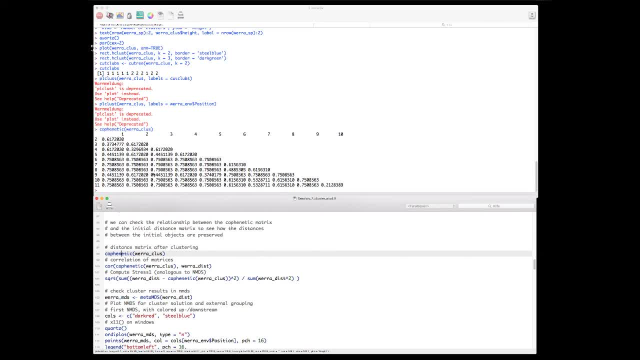 The Relationship Between The Objects. Again, It's Just A Matrix That Tells Something, That Provides Us Information Of The Distances Between Objects, And You Can. 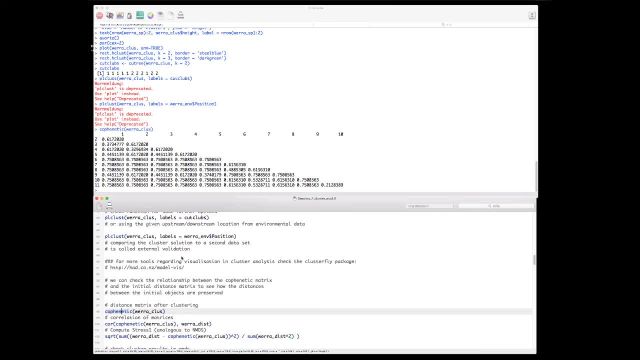 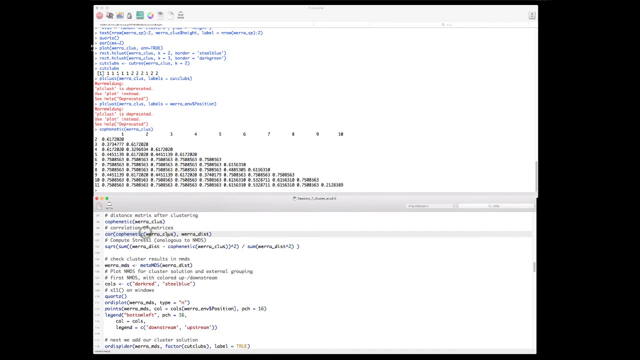 See That Based On The Cluster Solution Here, That With Two Groups And The Average Linkage, Then We Look At The Correlation Between The Initial 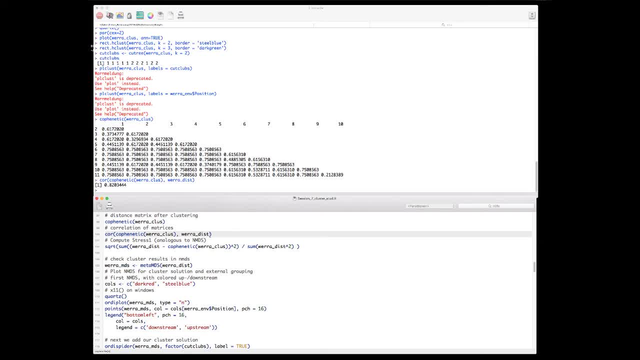 Matrix And The Co Phonetic Matrix And We See That They Are Correlated Relatively. That Is The Same Measure As For The NMDS From 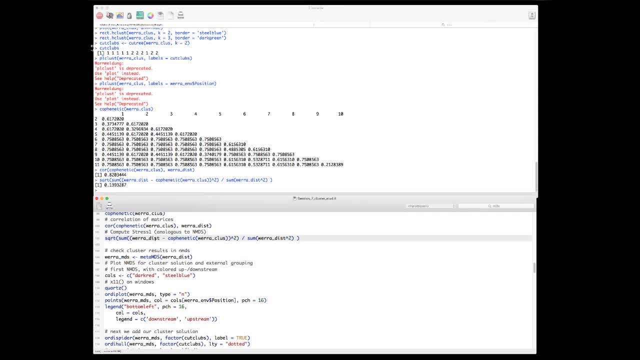 This Matrix, This Is Shown Here And We Had, We Would Have Stress Value Of 0.14.. And If You Remember The Cluster That Have 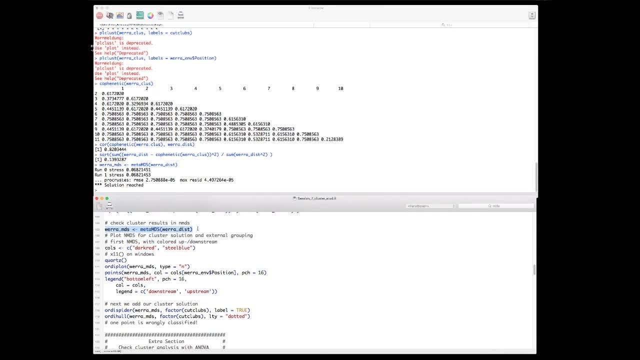 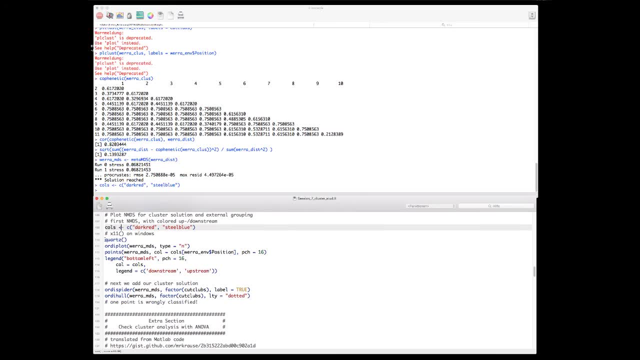 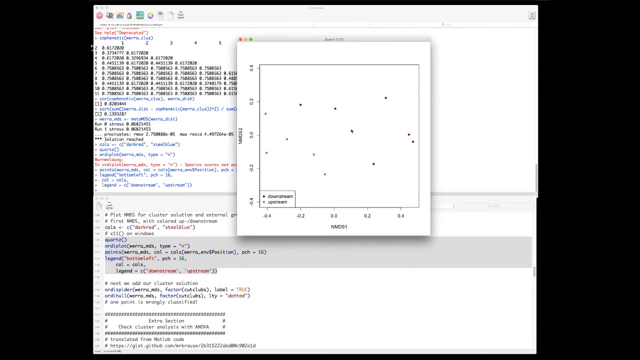 Resulted In An NMDS. So We First Conduct The NMDS, Then We Define Some Colors And Now We Plot The Results. This Is What. 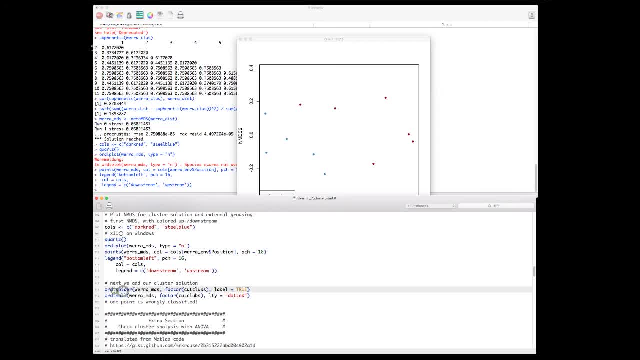 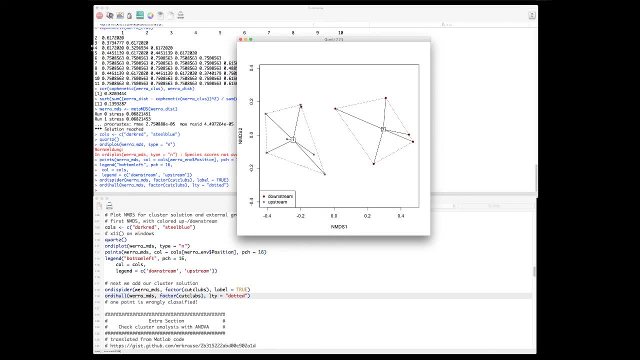 We Have Here And They Are Merged Into Clusters. You See That The Downstream Side Here Is Actually Put Into The First Cluster And 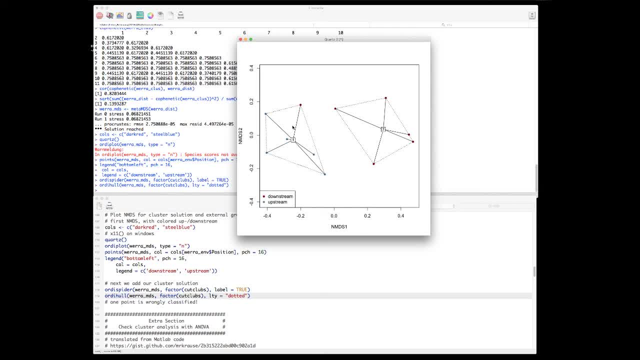 Our Clustering Process, Whereas The Other Sides You Never Or Rarely Have This Clear Cuts. You Mostly Have Gradients And Whether This Downstream, 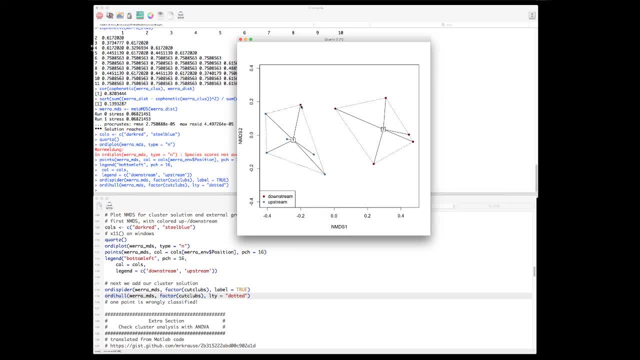 Side Is Really A Downstream Side. It's Actually For Salinization Of A German River. It's Probably Upstream From The Salt Discharge. So 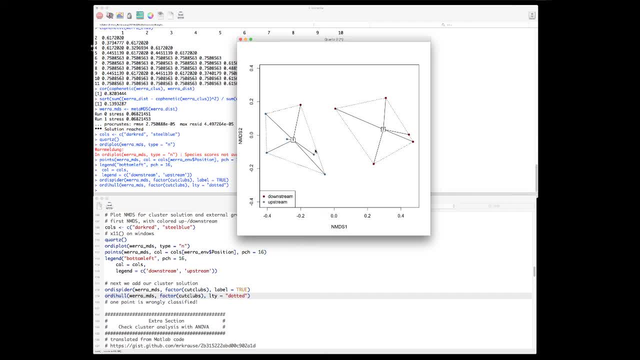 You See, That's Probably. The Communities Are Still Relatively Similar To The Upstream Side And This Can Be Due To Ecological. So This Point. 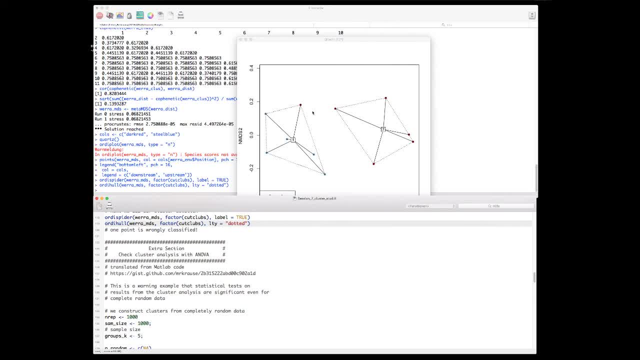 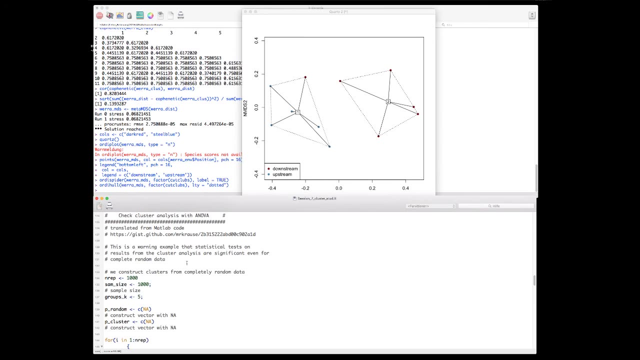 May Be Wrongly Classified From Statistical Point Of View, But, On The Other Hand, There May Be Reasons Why This Is The Case: Ecological Reasons, 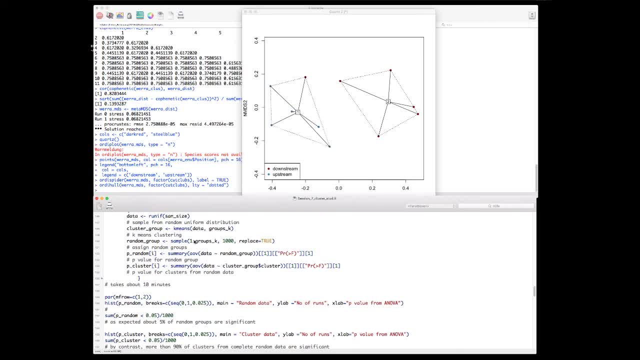 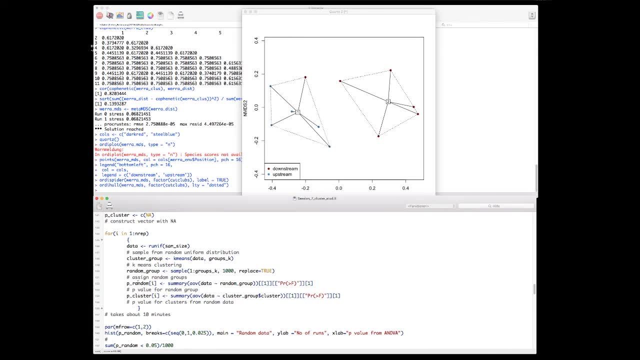 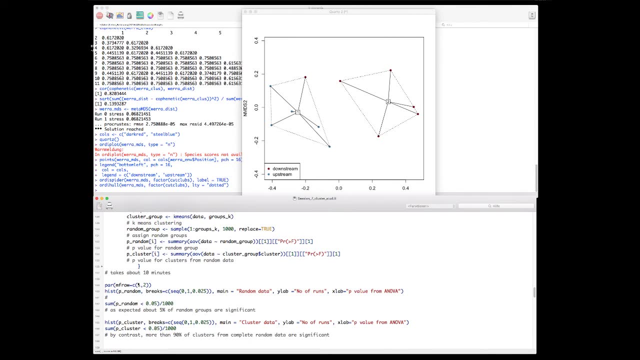 So I Have To See This Script, And This Part Would Probably Run About Ten Minutes, Or Five To Ten Minutes At Least, Depending On Your 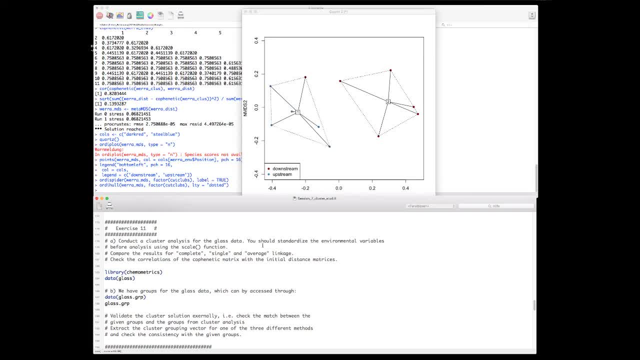 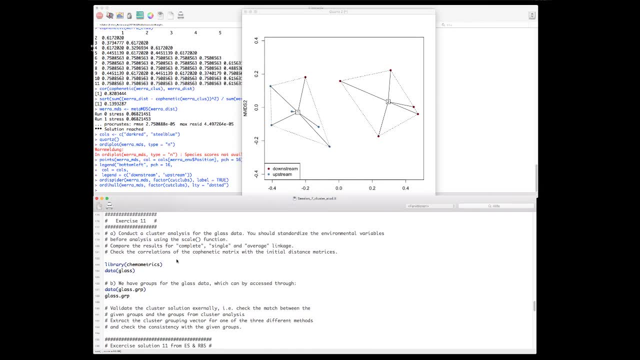 Computer Power And So Standardize The Environmental Variables Before Analysis Using The Scale Function. That Just Is The Aim That You Don't Have One Of. 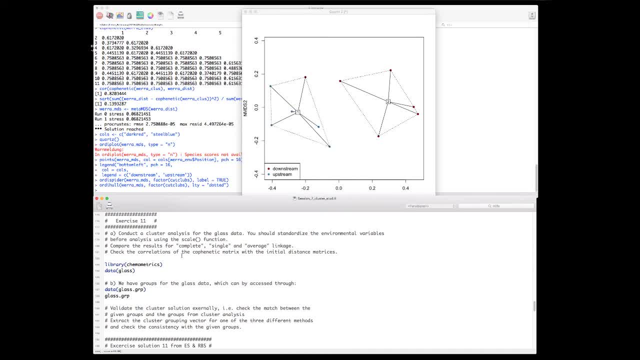 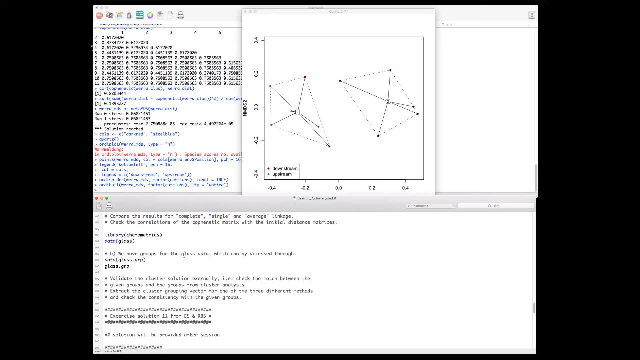 The Environmental Variables Dominating The Others, And Then Compare These Methods, Then Check The Groups. We Have Groups For The Data. You Actually Use Them. 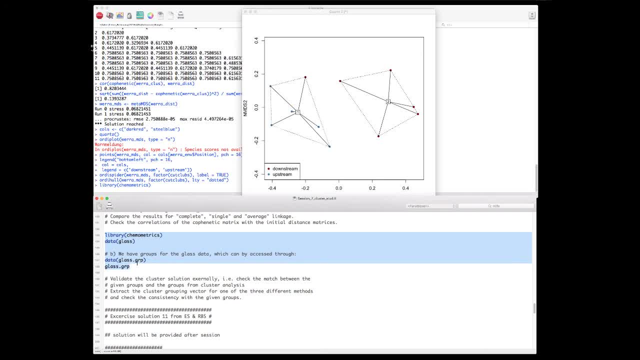 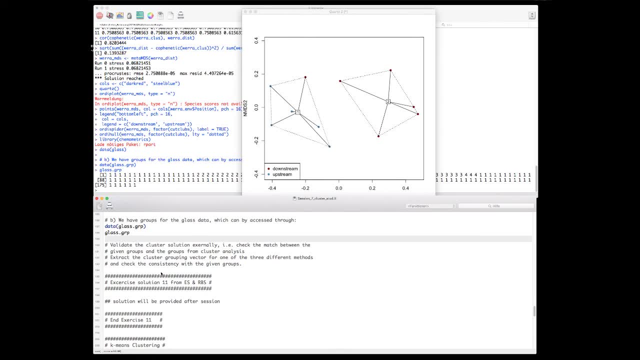 In A Different Exercise, And Then We Load These Groups And We Have A Data By What's Given, By The Data And You Could Obtain. 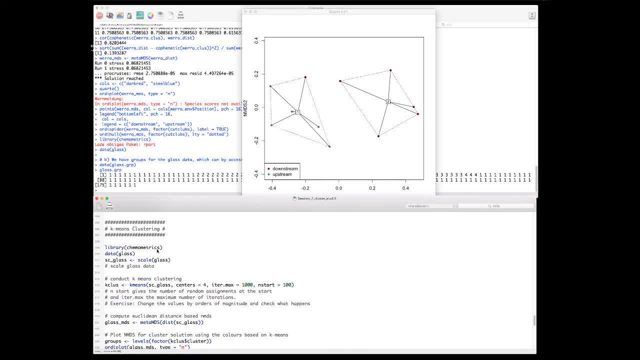 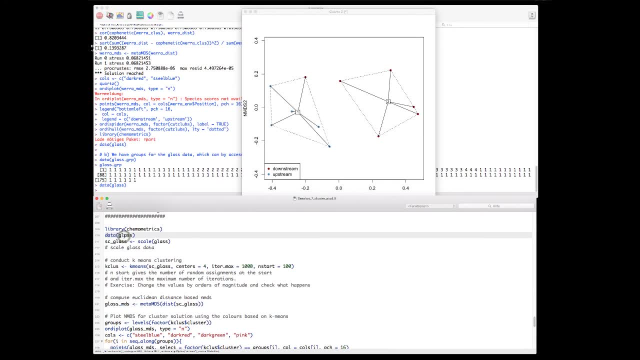 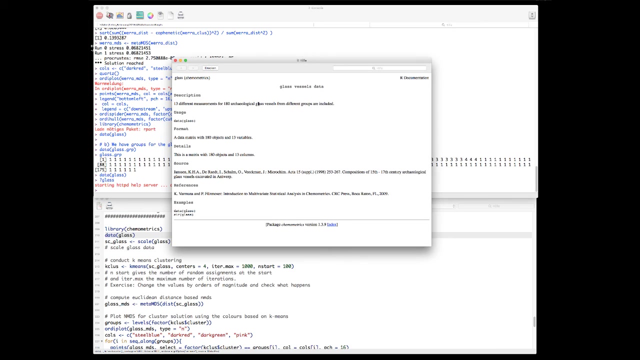 Exercise Solution From Us In The Other Script One. We Have Finished This Session, And Then I Move To The Question. Mark Contains Chemical Information On. 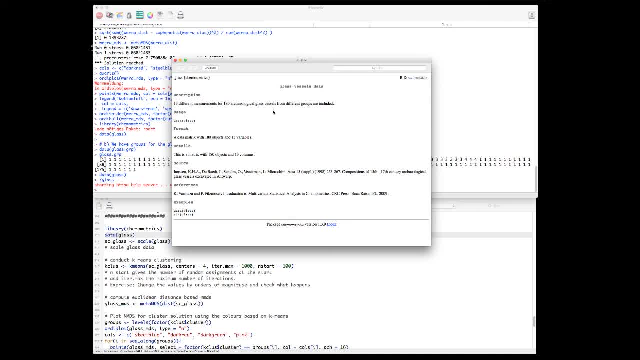 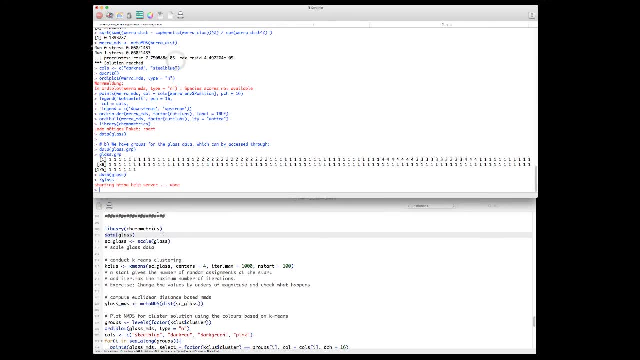 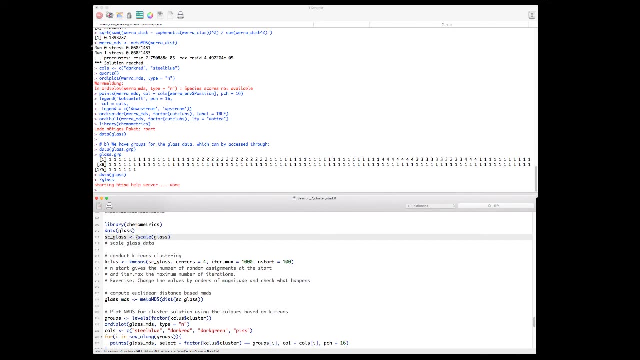 Archaeological Class Vessels That Have Been Found In And Work Around And Work, And The Question Is Whether These Are All From These, The 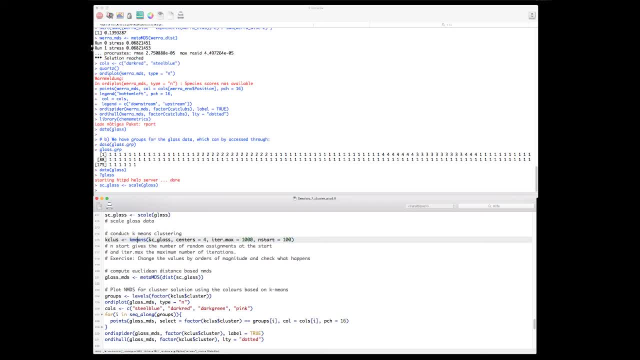 Data Have Been Established Or From You You Know That They Have Been Found On This Jail And Has To Be Found On This In This. 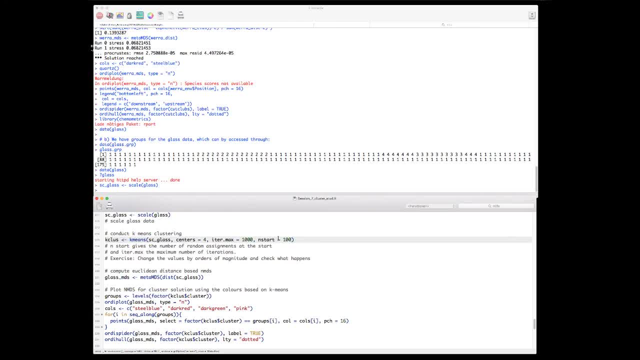 At the computer has to start with a certain cluster configuration and we start here with 100 different ones, and you could also change the values by orders of magnitude and check what have. what happens if you increase the number of starts? very often, much, much maybe if you increase this. 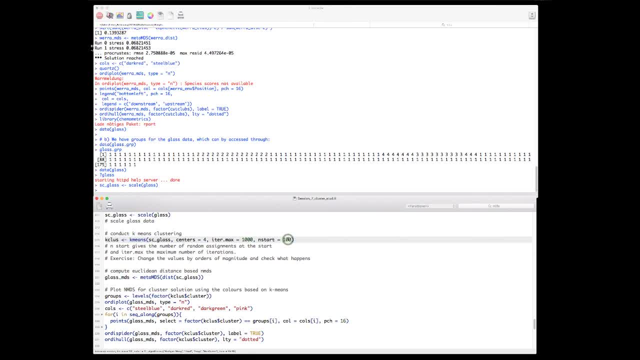 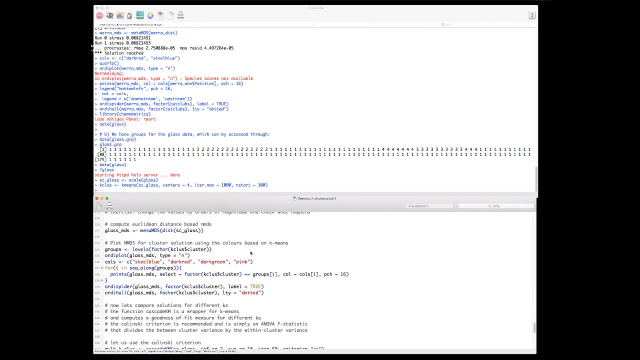 number um strongly. we'll also see that this takes much more time. just keep it very small at very limited time. here um now we obtain this cluster solution and we use this cluster solution in the visualization. first of all, we conduct again an nmds for display. 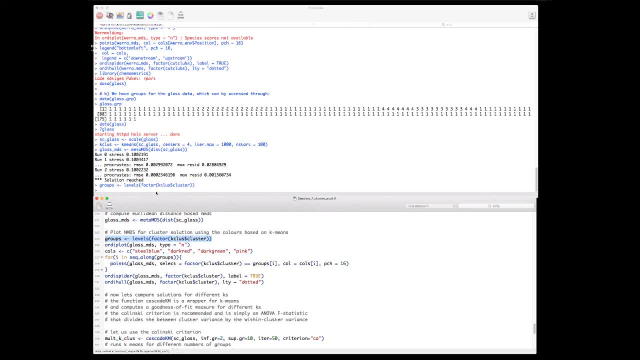 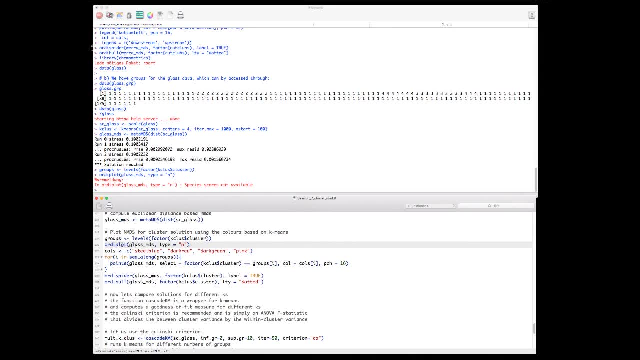 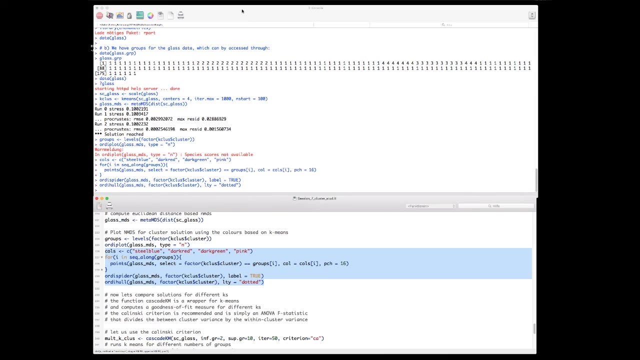 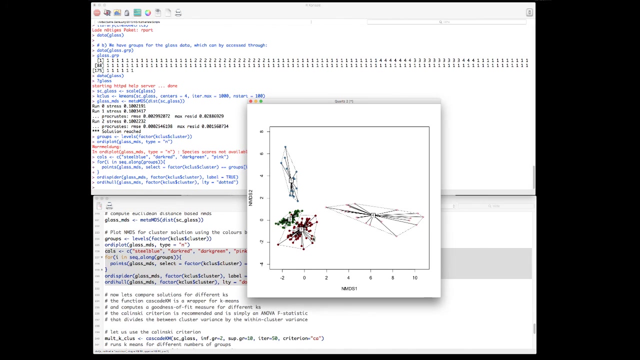 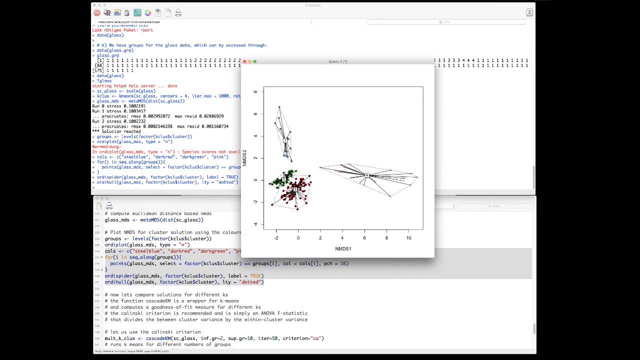 we use the groups from our cluster solution, k classes our cluster solution and we plot the data. so here's our resulting we know. what we see is that, on one hand, the points are given by the nmds and what we have displayed here is the cluster. 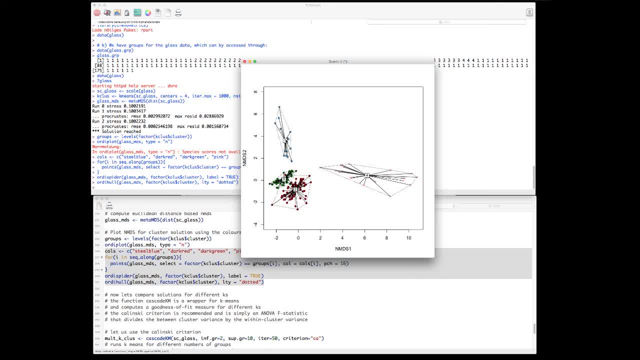 from the cluster solution. we have called here for four different clusters and we see that indeed most of the objects are classified as we would expect. we have the cluster four here, cluster one, but we see that actually here for these data points it's not so clear that you would have. 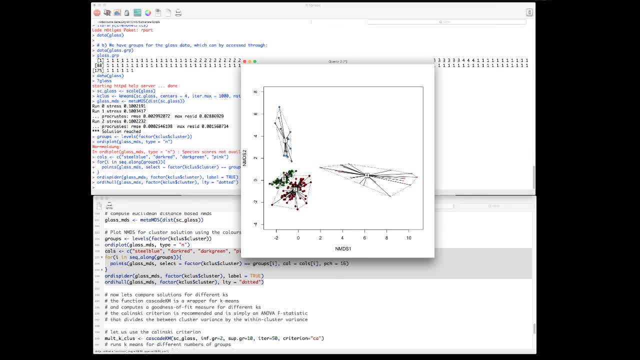 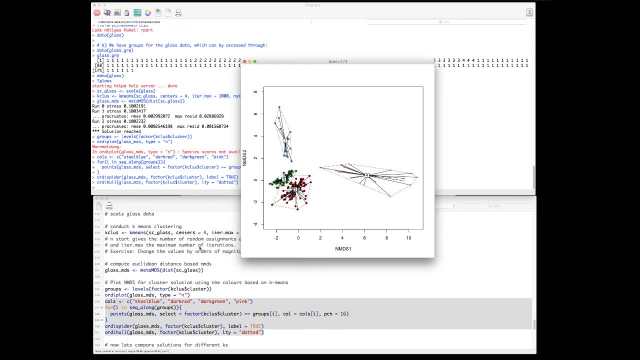 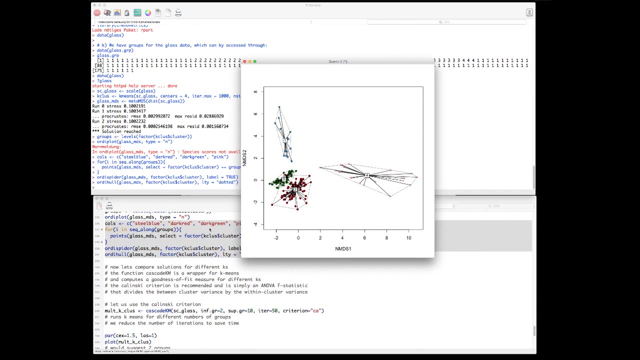 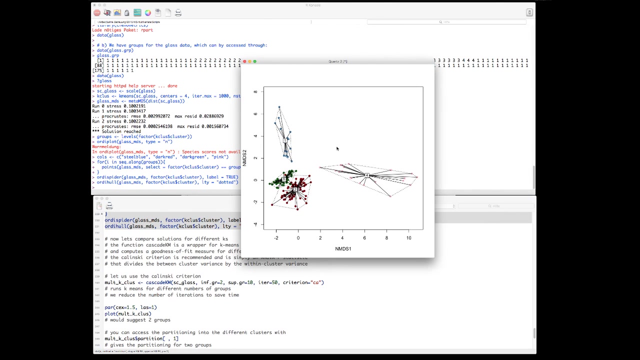 two different clusters, but it needs to be taken into account that, of course, the match of the real distances with the display displayed distances is not 100 percent. in an nmds, however, it's typically if you have no idea, or have not much idea of the data, it's, of course, difficult. 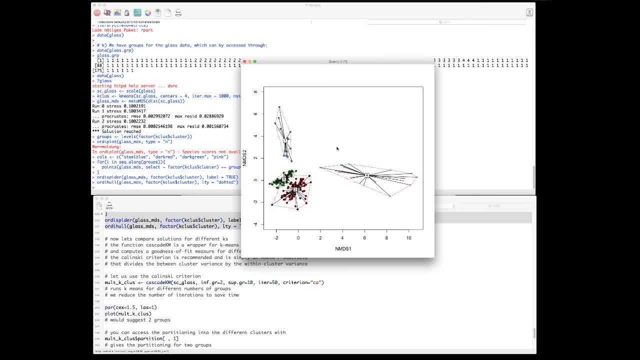 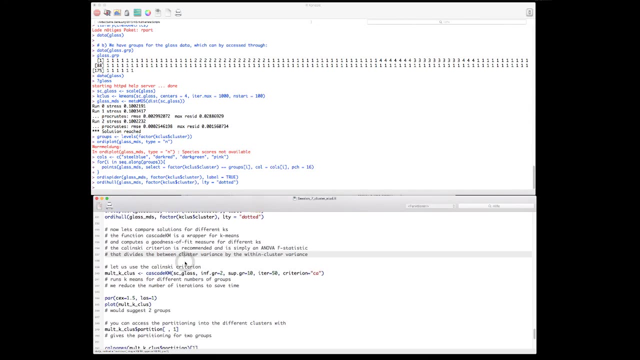 to come up with a number of groups that you would expect in the data set and therefore you. there are different criteria that have been developed to evaluate how the cluster solution compares to this, to a criterion, and one criterion is the so-called kalinsky criterion in the cascade. 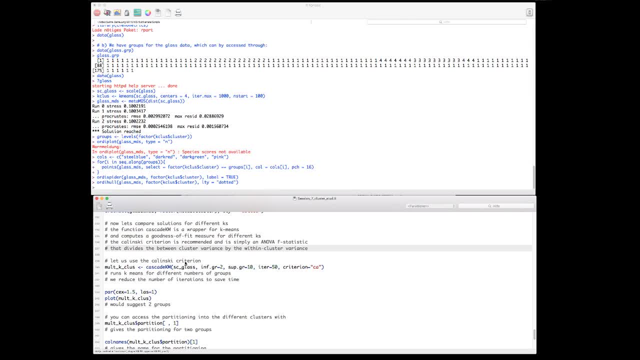 km function. this means this function uses different number of groups for the k-means algorithm and then calculates for each result the relationship between the between cluster, the relationship in the between cluster variants to the within cluster variants, and obviously the higher relationship of the with of the between cluster variants to the within cluster ranks is the better. 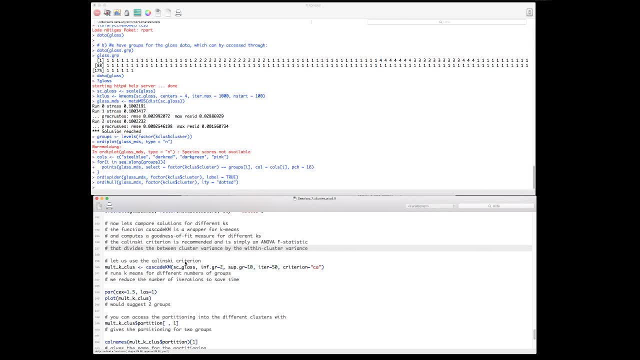 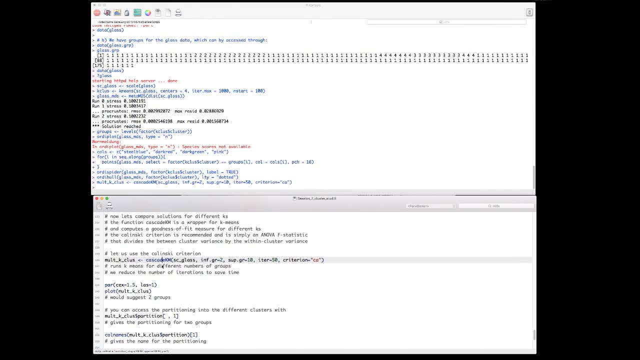 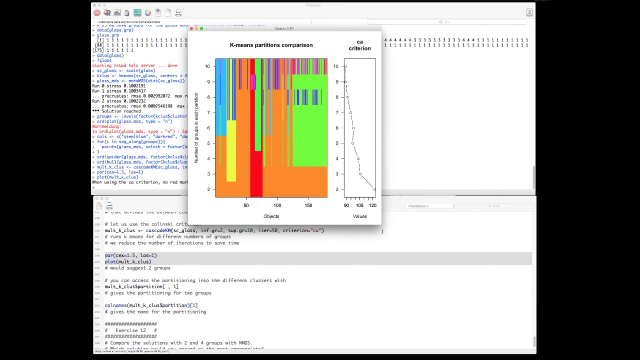 is the cluster solution. so you want to have low within cluster variants and very high between cluster variants. so we run this and what you see here, what is given here is- is the criterion that you use for evaluation and we can plot our plot the results. if we do this. we have here information on the k-means clustering that.